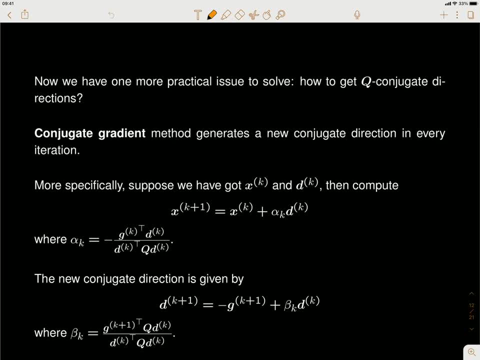 to conjugate the directions. But the problem is: how do we get these directions for the conjugate gradient method? We don't want to compute them in advance because, as we showed earlier, constructing them can be pretty expensive. We did one example for a 3x3 matrix. 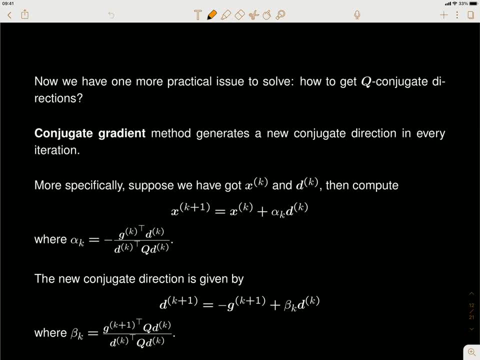 So the conjugate gradient method has a very clever way to get these conjugate directions during n steps, And the computation of these directions is much cheaper than the one we did before. So here this is how these conjugate directions are constructed along the way with the iterations. 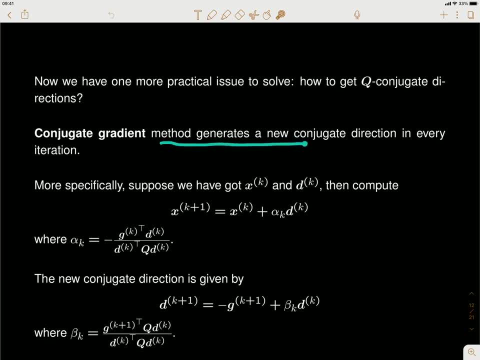 Now, as we said, we're going to show that the conjugate gradient method is going to generate the new conjugate directions in every iteration. And how are we going to generate them? Suppose we already have the xk and we already have the previous conjugate direction, dk, and then we know that we can. 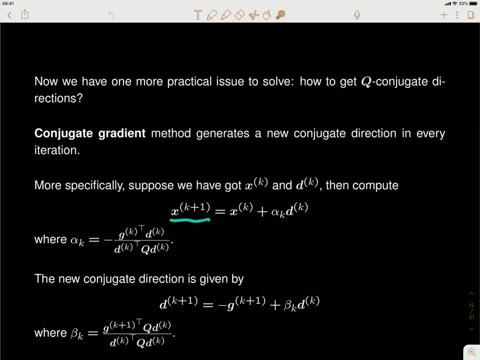 compute the next iterate xk plus 1, using this simple update. where this dk is a search direction, It's used as a search direction And this r for k is the step size. as we showed earlier, We're going to choose r for k to be this ratio. Okay, So scalar, which is the 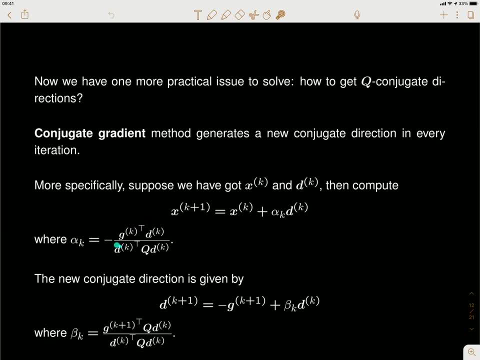 inner product of two vectors is a scalar divided by another scalar. So this is the scalar. This is going to be our step size. Okay, Now the problem is that now we get the new point and we're going to update the xk. 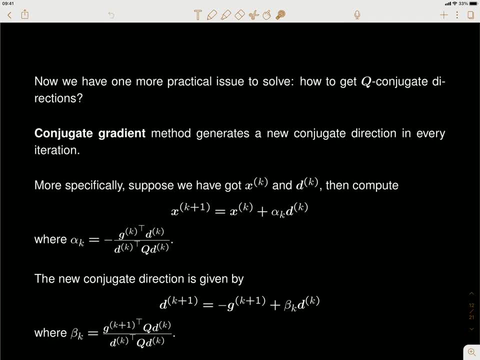 plus 1 using a similar formula to obtain the xk plus 2.. But to get that we need the next conjugate direction, dk plus 1. And the conjugate gradient method tells us that we can construct the new conjugate direction. 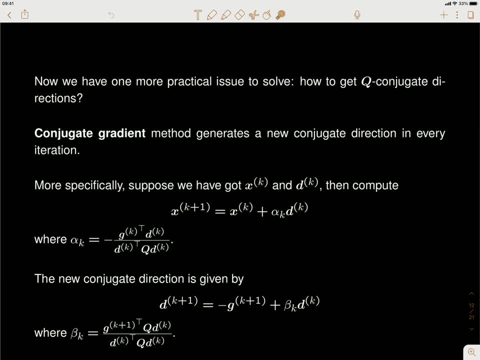 The new conjugate direction, dk plus 1, using the previous conjugate direction- This is where you came from- to get the xk plus 1.. And once you get the xk plus 1, you compute the gradient of f at this new point And that is the gradient, that's the gk plus 1.. So 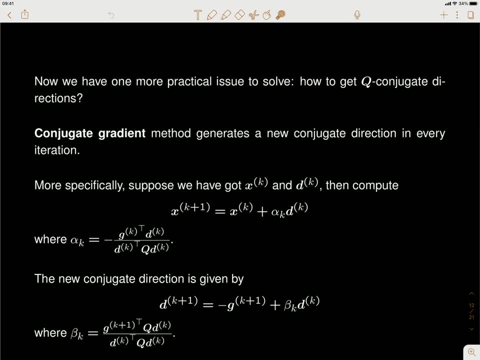 the next conjugate direction is a linear combination of the new gradient We just computed And so now we can start to 0.. Here you can see we deuxième nutr pendant of f at the new딱 plus 1, and the previous conjugate direction And the combination coefficients is the one. 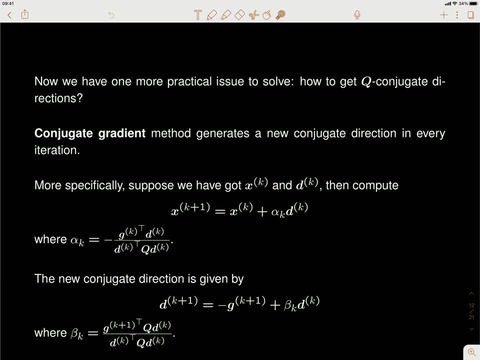 here and this beta-k here, And this beta-k is said to be this: Okay, This beta-k is different from the one that we used to prove the convergence of the basic conjugate gradient algorithm. So this is a different beta-k And this beta-k is used to make this combination of gk plus. 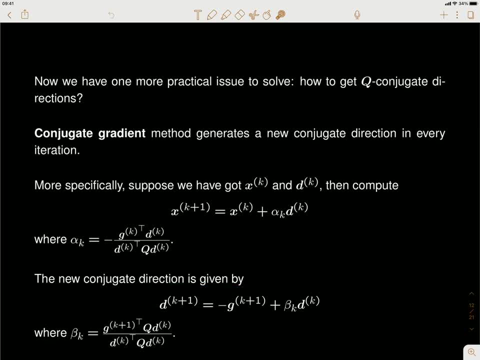 and dk to get the next conjugate direction. So now you can see if this is working. then we don't really need to follow the example we had earlier to construct those dk recursively and every new dk plus one is going to be q-conjugated. 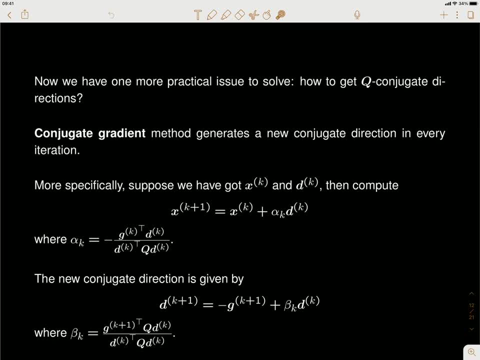 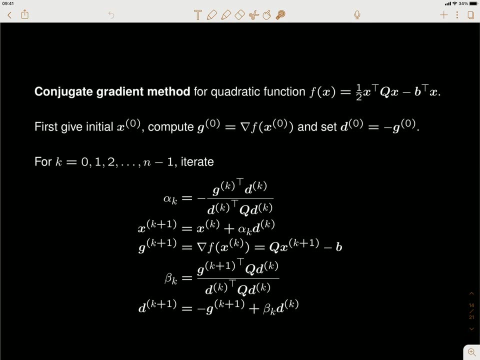 with respect to all the previous ones, which is very expensive. Now, the update of this dk plus one is very simple. You're just doing this, okay, Okay, so now let's see how this is going to work. Again, we're considering the quadratic functions first. 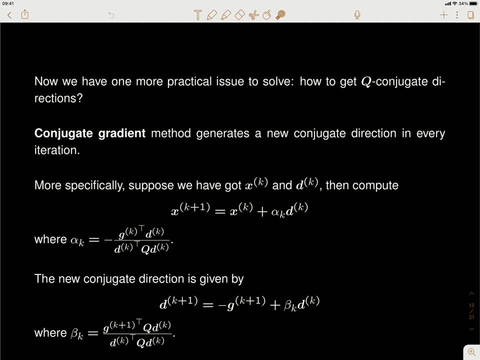 Remember that we're focusing on quadratic functions and that is also the reason why this r for k can be chosen in this closed form. is this closed form because that is the steepest and the steepest descent step size for quadratic functions. 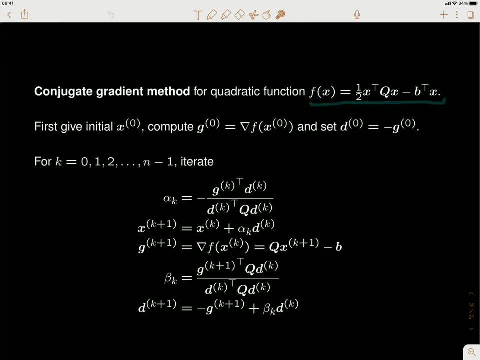 Now this is our quadratic function, where q is positive definite, And then, given the initial x naught, we can compute the gradient f at this x naught, and that's our g zero, our g naught, And then we'll just set the first conjugate direction. 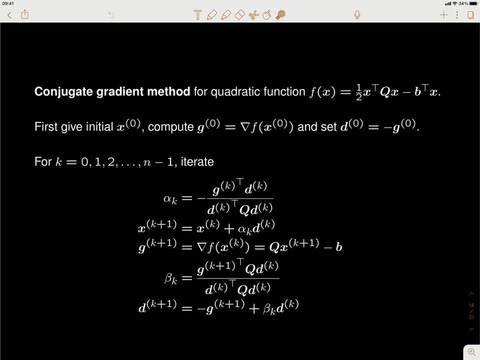 as a negative gradient, negative g naught. That is the gradient. negative gradient direction is going to be our first conjugate direction And then, starting from there, we can compute the step size You use that to update. So this is exactly the same step size we used earlier. 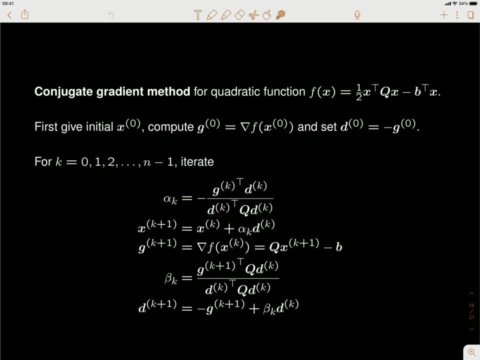 I'm not going to be expand this more. And then, once you have the step size, you have the current x zero and d zero, And then we have the d ph zero. Now we can get x one. okay, But in general, 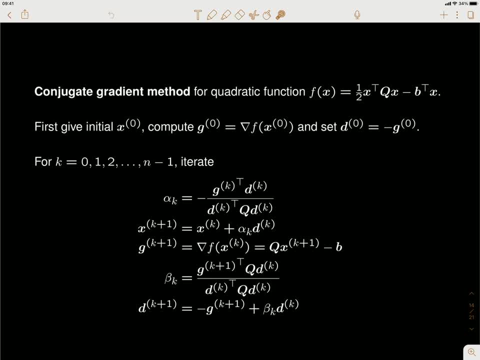 you want to create that, look to get pa 1,, x2, and x3.. we have xk and we can compute the gk, and then we're going to update the dk, and update the dk using the previous former, and then we can, we can do this step. okay, so now, for now, you just 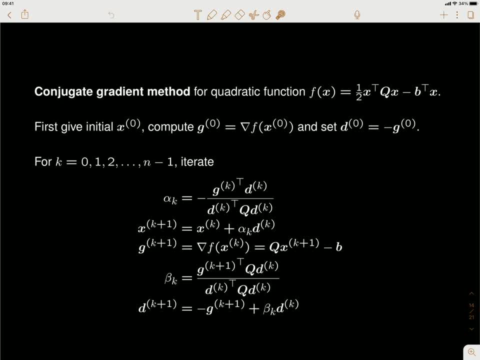 think that we start from k equals zero. then, as we said, we compute alpha zero and all we need, uh, all this g zero and d zero and which we already have- g0, d0, this okay- and then compute alpha zero and then we have x1 and once we got x1, we can compute this. 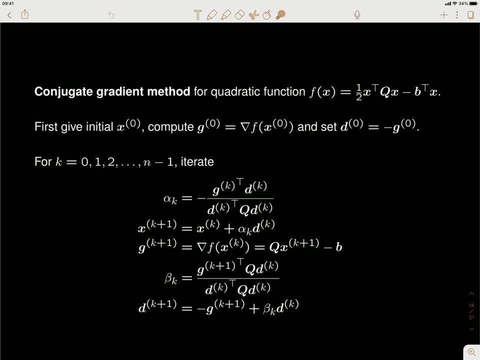 we can compute this gk plus 1 or g1, and then, once we have the g1, we can compute the beta beta 1. uh, again, Again, on the right hand side, everything is known. And then, once we have the beta one, we can update the descent direction to get the new. 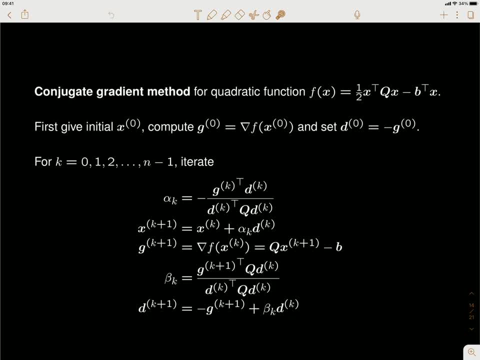 conjugate direction, to get the new conjugate direction which is also our descent direction. And now you can see, but after this step we can get the d1, x1 and g1. And then we're going to increase k by 1, and k will be equal to 1 now, And then we can compute. 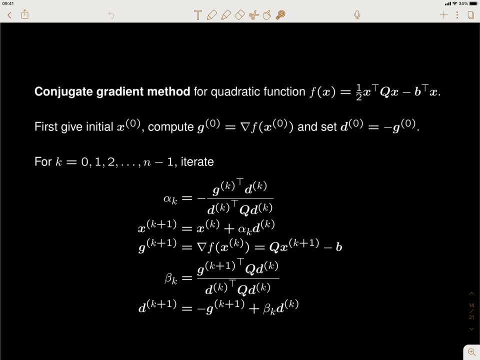 this alpha 1, then x2, g2, so on and so forth, Okay. so, for each iteration, we're going to do these steps. Okay, we're going to do all these steps, Okay. So before we move on, let's first see what is the computational cost of this algorithm. 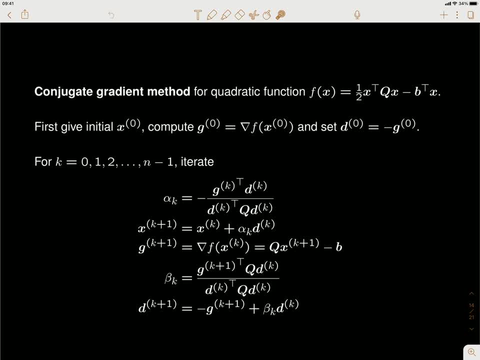 Okay, We said that we're going to iterate this for at most n steps, And this is because this algorithm actually generates these conjugate q-conjugate directions, And we know that in this case, the algorithm should converge within n steps. 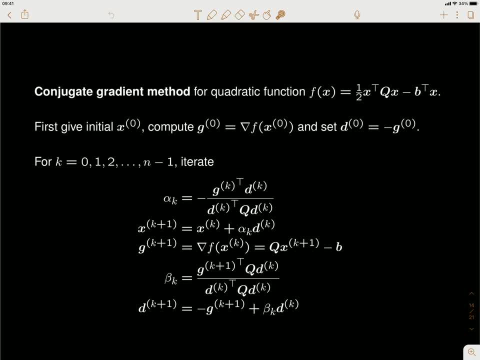 So we're going to only run it up to the x-hand. It's supposed to give us the true solution. Okay, so the thing that is still pending is why this is going to be a conjugate direction. That is something we're going to show later. 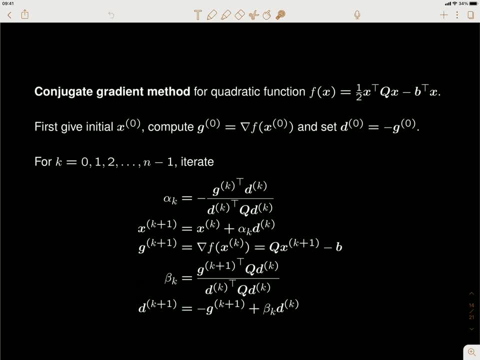 But suppose this is true And let's see that we're going to run this iteration for n steps and for each step how much computation we need. Okay, as you can see, to compute this alpha k. to compute this alpha k, what I will need is a inner product of two vectors and 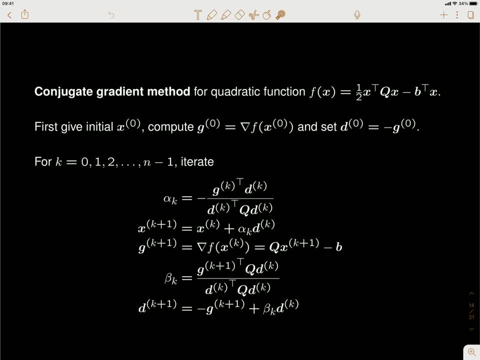 to make an inner product of two vectors, two n-dimensional vectors. we need to make n multiplications by component-wise multiplications And then we need to sum them together, which requires n-1 summations. So the inner product of two n-dimensional vectors requires: 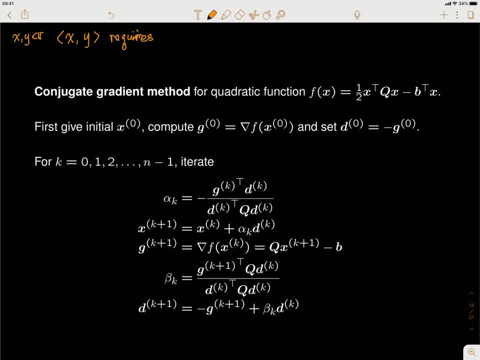 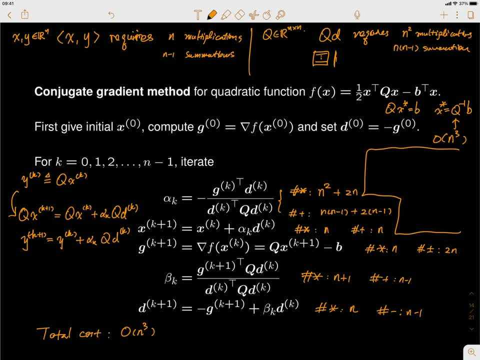 So x, y, they're all n-dimensional vectors. So x, y, they're all n-dimensional vectors. So remember, in practice most of the scientific computing problems can be written as a big linear system. AX equals to- let me use another notation: AX equals to vector C. 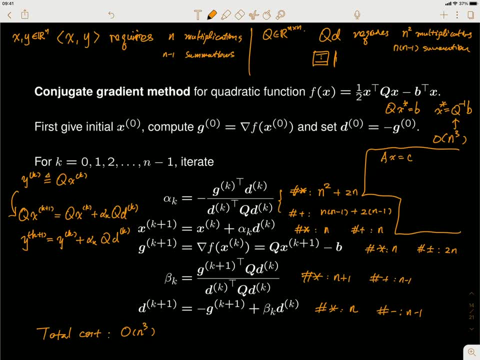 And this A is extremely large. This A is extremely large. Well, as we said, this A can be hundreds of thousands by hundreds of thousands. So the problem is that this A can be hundreds of thousands by hundreds of thousands. actual purpose, or the original purpose to solve this x is to b for x and uh. instead of doing this, 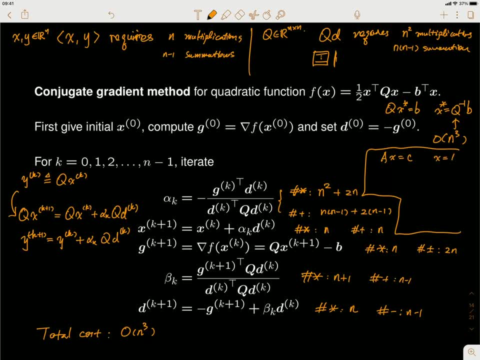 we can. you know that. you can just say that x equals to a inverse times c. let's say a is square matrix and the invertible, and it will say that my solution is just this. well, uh, in practice that's not what we people do. so what actually do is done is that the uh, you consider the. 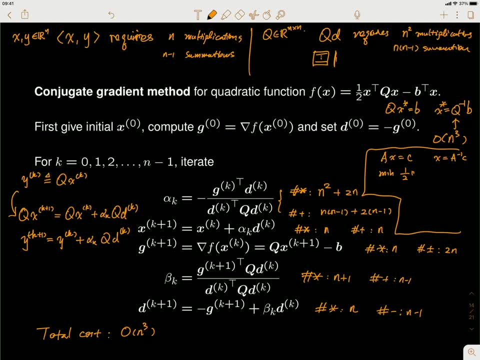 minimization problem of this ax minus c square, and apparently this is non. this is objective. function is always greater than equal to zero. if you do have a solution such that ax equals to c, then the minimizer should be that solution, right? the minimizer of this problem is the solution. 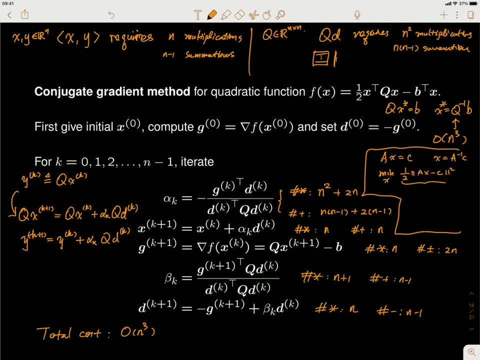 of ax equals to c. but you look at the objective function here. this is our objective function. if we break the square, we'll see that this is nothing but the one half times x. transpose a. transpose x. a transpose ax minus c. transpose ax plus one half times c. square. 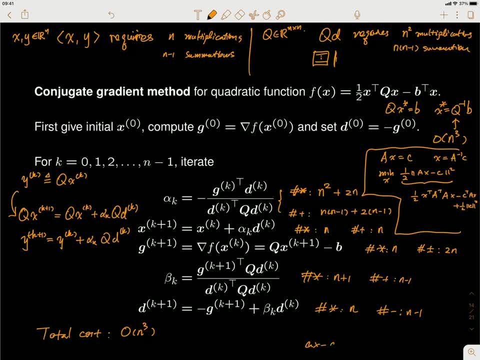 okay, so this is basically like a times x minus c and you take the square, you have the a x square minus 2c, times ax plus c square and you have one half, then just everything divided by two, and this ax right now is the vector ax and this square of this vector x, and that is just a. 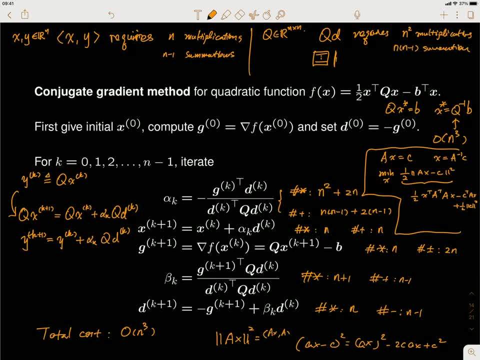 you know it's just the inner product of ax and the ax, and this can be also written as ax, transpose times, ax. okay, and you try, you put the transpose inside, it will be giving you- uh, this will be giving you- x, transpose, a transpose ax. that is what this term comes from and the interacting term is this, so it's like this: 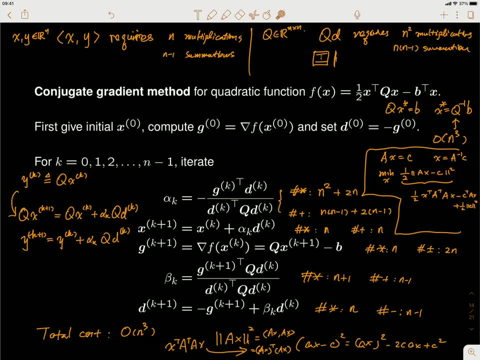 c times ax and then you have this. this is a constant. once you have the c, this is constant. so this is a constant which doesn't affect you, the the choice over minimizer, and you can see that you can't use all the arguments because you can't do it regardless of any function, because 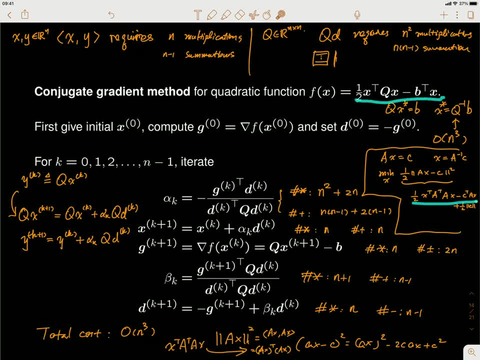 this right here. uh, we have one más, and this one is now true. so this is the unilaterality NF of either of the variables. x is even what's about n, because there's no single denominator of c�ago, plus the Question what's very important in this user. 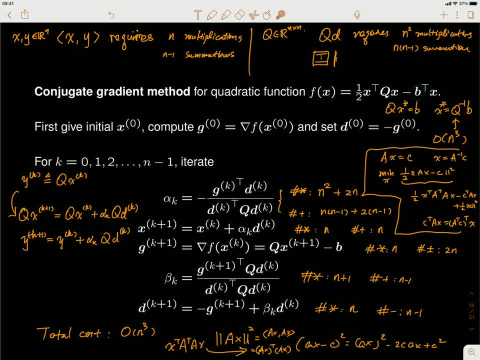 here is the b. okay, so this, as we said, this a transpose a is the q matrix and this a transpose c is this b vector. okay, so it's like you're given this matrix, you have the a, c here, so you can construct this matrix and this a, this a times c, or this a transpose c. 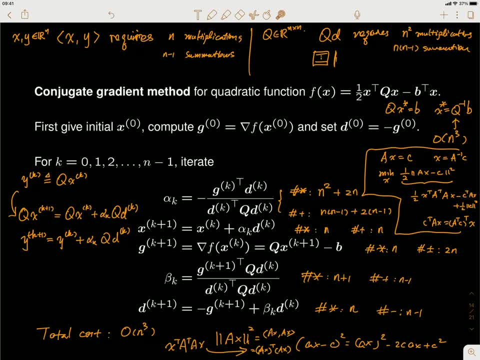 as the vector and you are just minimizing. you're minimizing this. so minimizing the least squares is the same as minimizing this quadratic function and it's the same as solving this linear system. okay, so a conjugate gradient. this conjugate gradient method was actually developed. 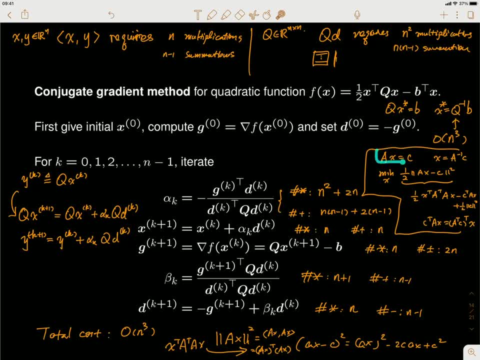 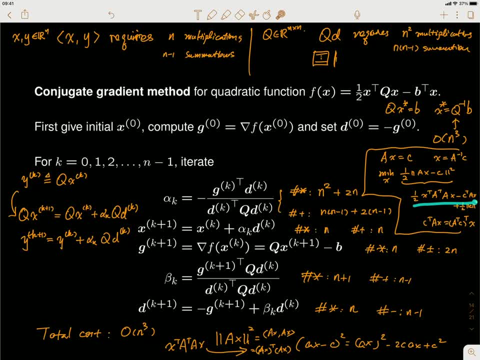 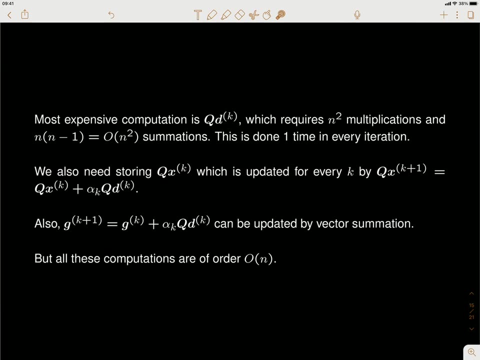 we just saw in this, in this optimization text context. okay, so now you basically give you a motivation why we study conjugate method. it is still the state of art, even it was divided about 50 years ago. it's still the state of art. it's still the fast algorithm that one of the 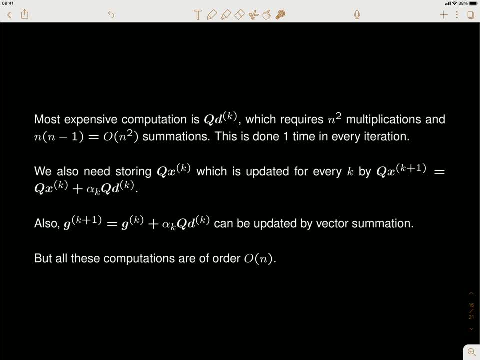 fast algorithms. we see that we use in practice. okay. okay, here is just a summary of summarize summary of what we we had in the previous slide. we said the most expensive computation is qdk, as we showed now. it requires n square modifications and also some summations. but we said 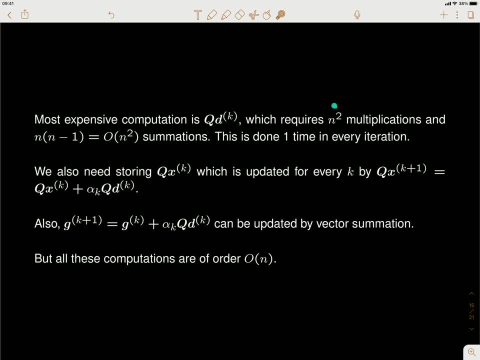 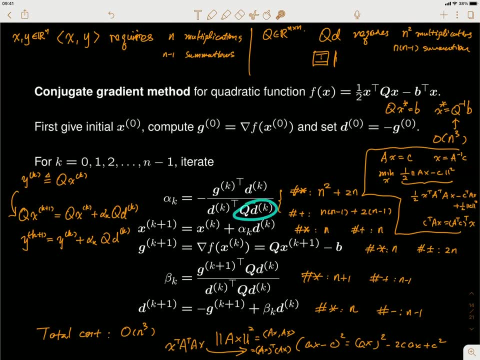 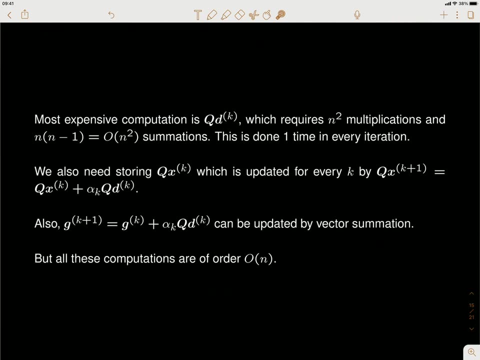 this is the dominating part. again, for each iteration, this is done for one time only. okay, although it appeared, the qd, the qdk appeared several times, but actually we only need to do this once and then this is the one thing that we mentioned to: to save the, the, to save the qdk. 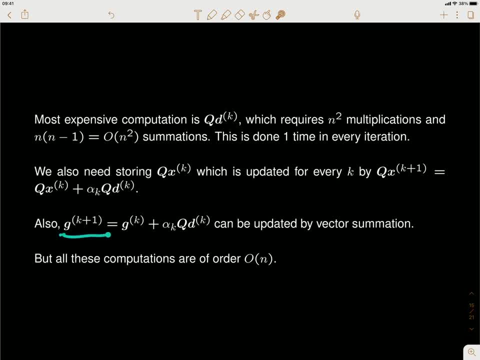 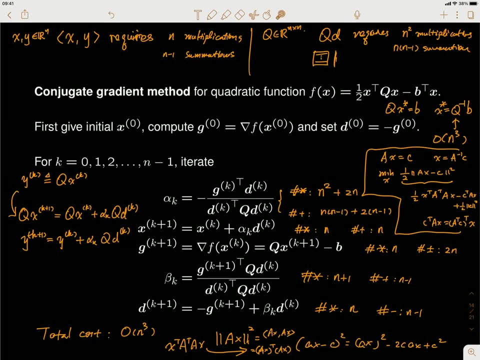 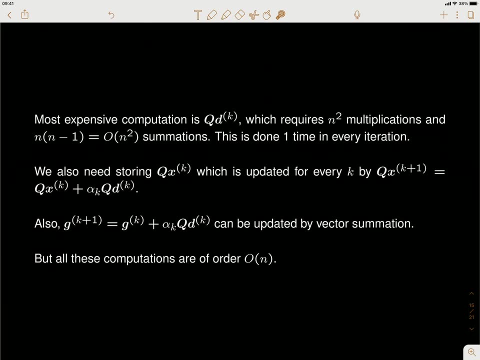 for computing the gk, since the gk, um, since it's not gk, it's this one. yeah, this gk is actually updated in this way because the, because the uh xk, because of this step. 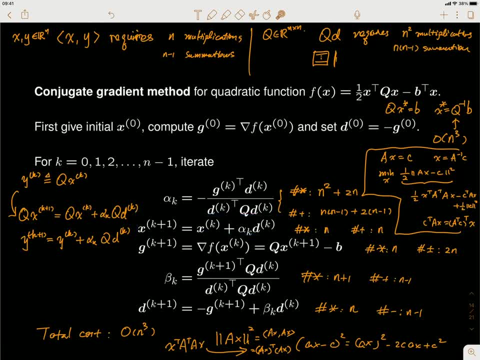 and we said this step: you can modify the q, xk, q on both sides and we get this. and instead of really storing this yk plus one, we can just subtract the b on both sides for this uh equation, and we know that this part will give us just gk plus one. 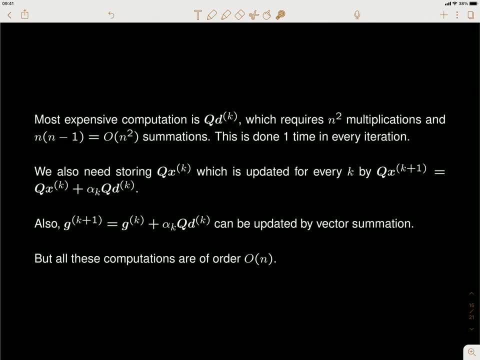 this part just give us the gk. so actually we can just directly update the gk plus one using this: okay. gk plus one using this, uh, instead of storing another y, okay. this is also some small trick that can reuse this thing to compute it. 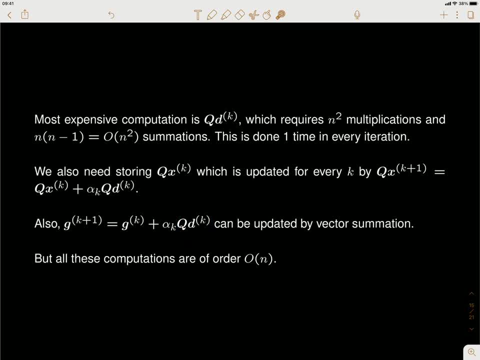 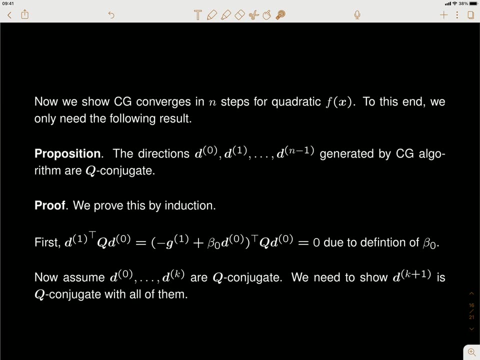 so the only thing that we, the most expensive, the only expensive thing we computed is this: qdk for each iteration okay, but all those iterations, only this one takes n square, all the others should be just n okay. so now, finally, uh, we need to show that, uh, the, uh, the beta, oh sorry, the, the dk's we constructed along the way of. 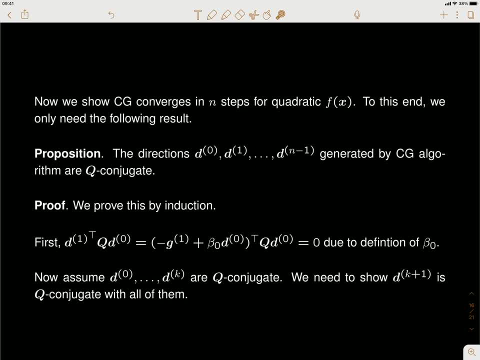 conjugate gradient method are actually q-conjugate. okay, um, so that's the proposition we're going to give here. the directions d0, d1,, so d-minus, were generated by the conjugate conjugate gradient method. uh is, are this q-conjugate? 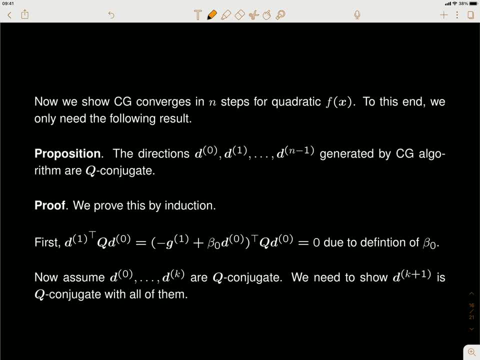 okay, so remember that. what we need to do is to show that for each dk plus one, it needs to be q-conjugate with all the previous uh dj's, so I need this to be zero for all dj's, from zero one to k to k. 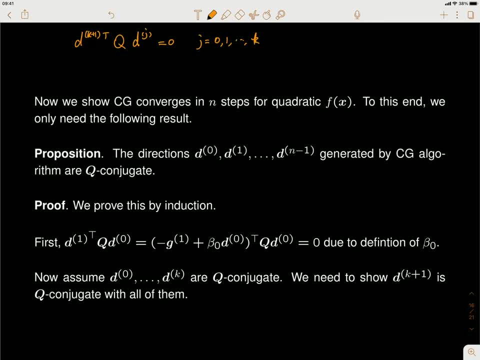 okay, I need to show that for each dk, plus one. show this is true for every k. Okay, and again similar as before, I'm going to prove this by induction, For first to show that d1 is q conjugate with d0,, d0, and then we make this as a. 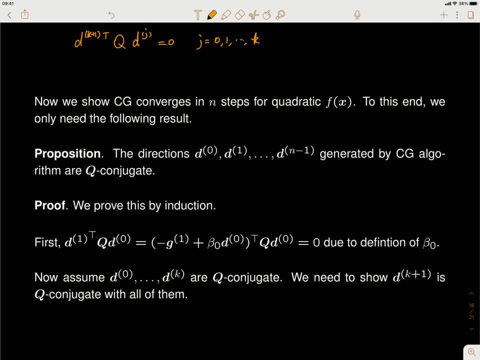 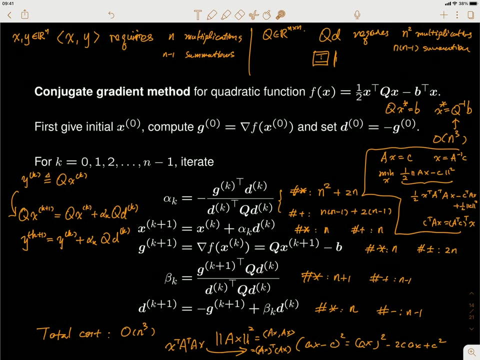 hyper induction, hyperphosphate, and then prove the next decay. Okay, so for the first one, we need to show that this is equal to 0. And the reason why this is true is because the d1, remember that the d1 was updated according to this last formula, So d1 should be equal to. 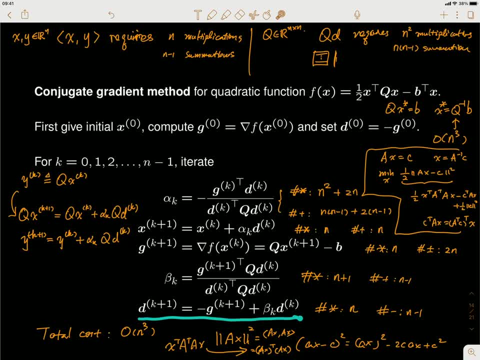 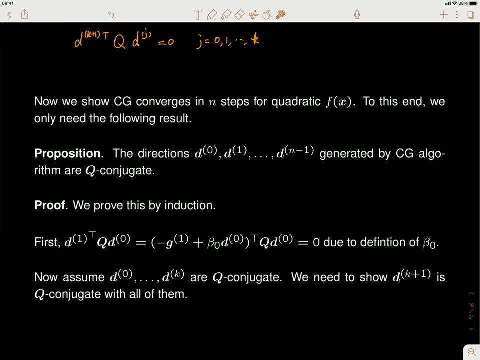 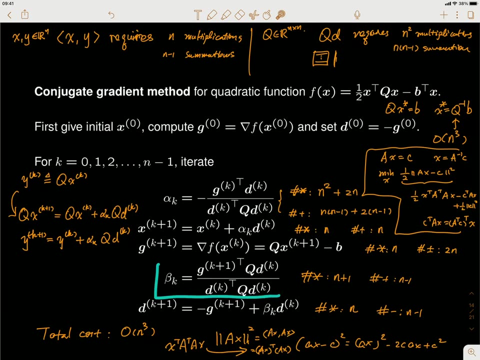 negative g1 plus b0, d0.. Okay, so that's this. Okay, and why this is equal to 0?? It is because of the beta 0 we chose. We set our beta 0 as a scalar As a scalar, Okay, and this for beta, for k, equals to 0, on the right side, we just have g1,. 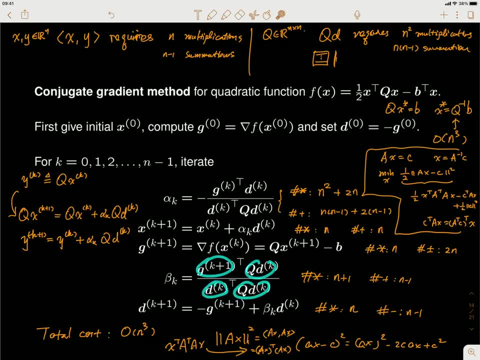 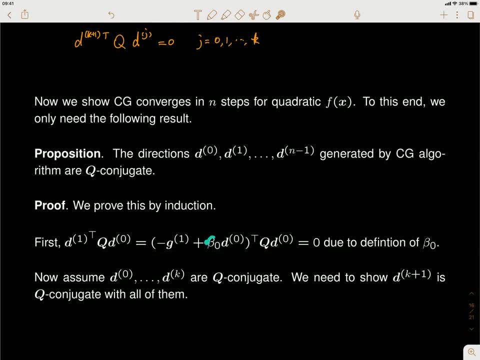 qd0, and denominator is d0, qd0.. And that is exactly the one that makes this quantity equal to 0.. Okay, so that's the choice for beta 0, and that makes it 0.. So we have the first one. 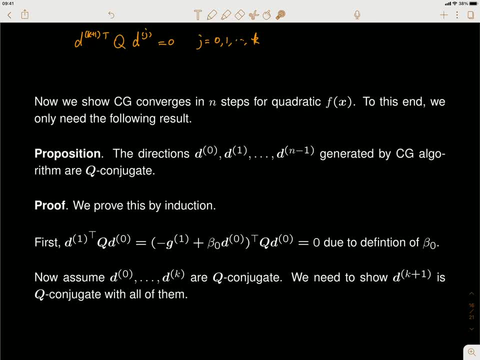 for reduction as a starting point of a reduction. And now let's assume, let's make the reduction hypothesis So assume that at the iteration when we got the decay, all the d vectors from d0 to dk are q conjugate. And assuming this is true, let's show that dk plus 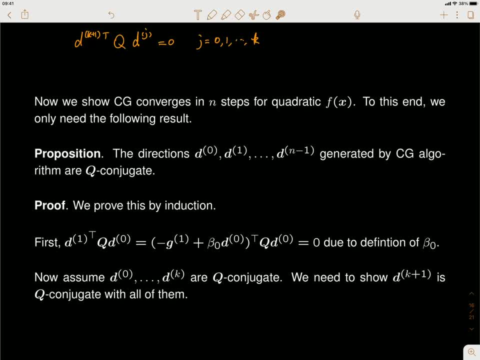 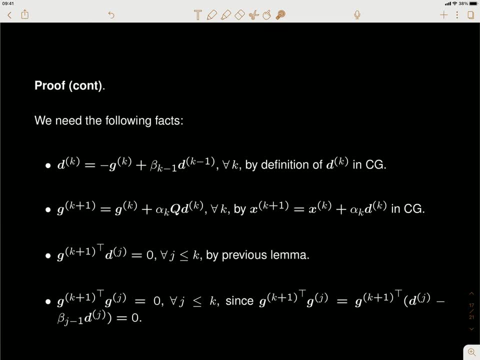 1 is q conjugate to all of them. Okay, and that is the one we're trying to show here. Okay, now let's see why this is true, And it requires several facts that we have developed earlier. The first one is the way we constructed the decay. Remember that we constructed the decay using the. 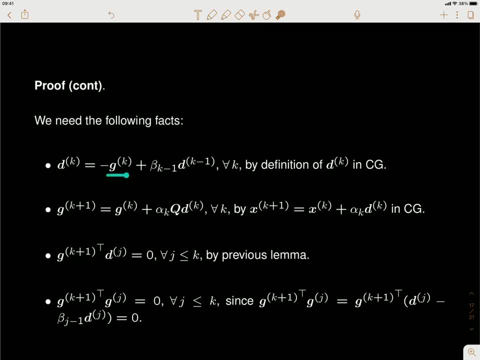 negative gk. So originally we have: dk plus 1 equals negative gk plus 1, and the beta k dk. But now I just decrease k by 1.. It's still true. So dk was related to the gk and dk minus 1 in this way. 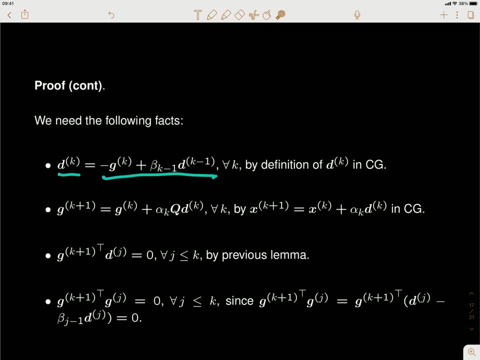 That's the one that we this definition for decay. So that's one thing that we know. The other, the second thing we know, is that the gk plus 1 is related to gk and dk in this way. Okay, and the reason is: we know that xk plus 1 is related to xk and dk. This is our updated rule. 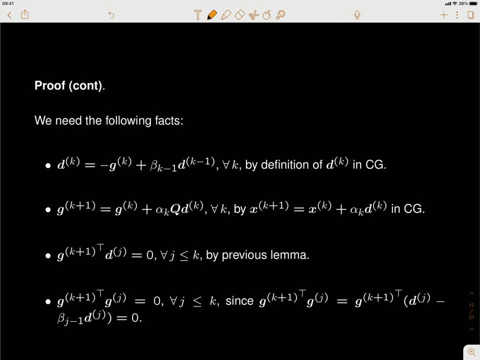 And then we multiply the q on both sides and subtract the b and we'll have qxk plus 1.. minus b, And on the right hand side we also have qxk minus b, plus this alpha k, q times dk. Okay, and then we said that this thing here is just the gk plus 1, and this thing is just the gk. 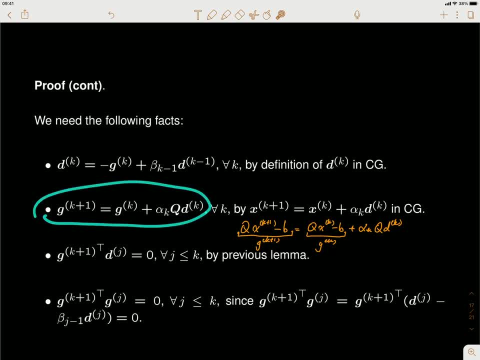 So that's why we have this, this one here. Okay, that's the second effect. The third effect is one of the lemmas we showed earlier. Each gk is perpendicular to the gk plus 1 is perpendicular to d0 through dk. Right, that's the one, the lemma we proved in the 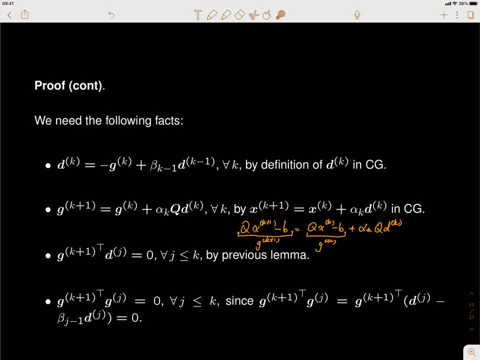 last lecture. So this is equal to 0.. And lastly, we're going to show that gk plus 1 is perpendicular to all the previous lemmas. So gk plus 1 is perpendicular to g0 through gk. And the reason for this is because remember that. 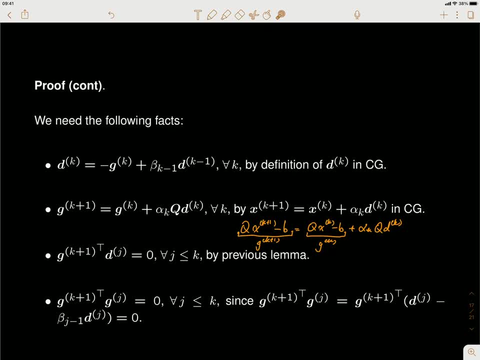 the dk. the gk and the dk are related in this way. this first way. So that means the gk is a linear combination of dk and dk minus 1.. So if gk relates to only as a linear combination of dk and dj and dj minus 1, but j is less than equal to k, 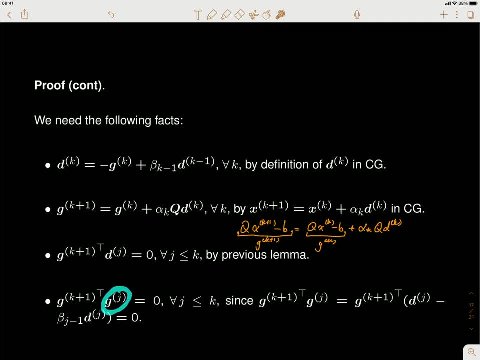 So that means this one will involve will be a linear combination for some d's and up to dk. Okay, the last one is this one. the last one is gk and it can be written as dk linear combination of dk and dk minus 1, like this one here, using this: 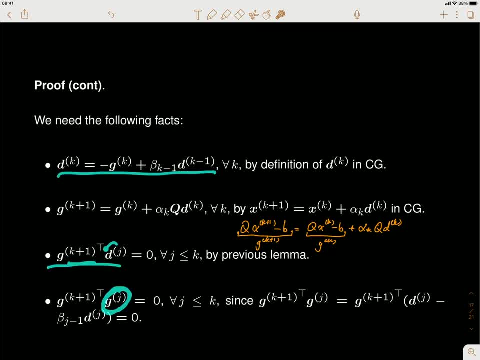 And but we know from the third one here that the gk plus 1 is perpendicular to all the dk's up to all the dj's up to j, equals to k, And this is written as a linear combination of those things, so it is still perpendicular to this. That is why this is also equal to 0.. Okay, so not only this. 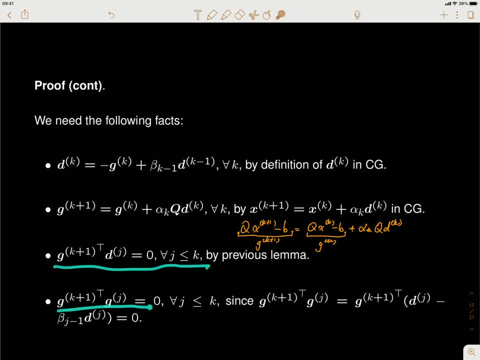 is equal to 0 for j less than equal to k, but also this equals 0 for j less than equal to k. Okay, so these are a few facts. we need to prove the next for the next, the dk plus 1.. 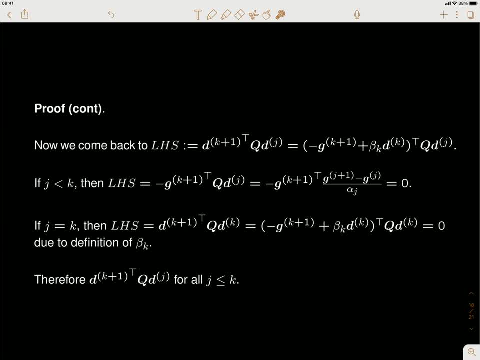 Okay, so remember that we're going to. we want to show that the dk plus 1 qdj is equal to 0 for all the j less than equal to k, And by this we can show that dk plus 1 is perpendicular or is q-conjugated. 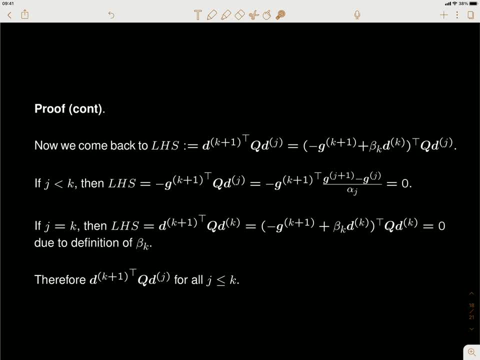 to all the previous dk's. Okay, So to show that, let's first recall that the dk plus 1 was updated by using the gk plus 1 and dk in this way. This is how we update the dk plus 1.. 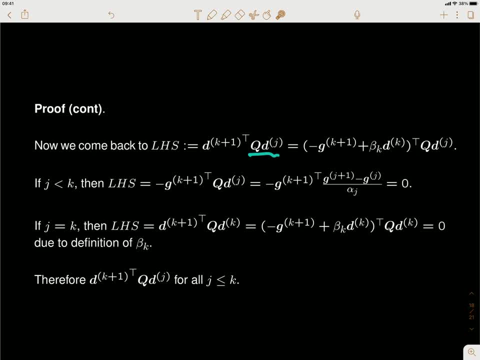 And to show that it's q conjugate of dk with dj which is need to multiply this to q dj and see what happens to this. So there are two cases: Either that j is strictly less than k or j is equal to k. So there are only two possibilities. 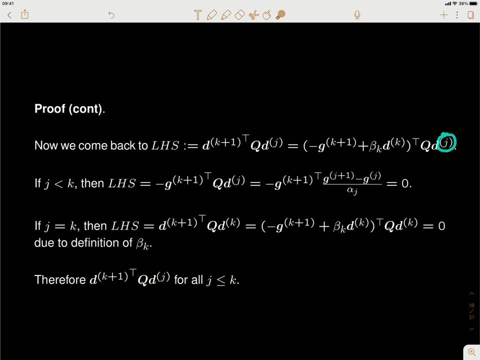 So for j is less than k, that means j is 0,, 1,, 2, up to k minus 1.. What happens is this quantity here is multiplied to the q dj. But q dj, as we showed in the previous one, the q dj is 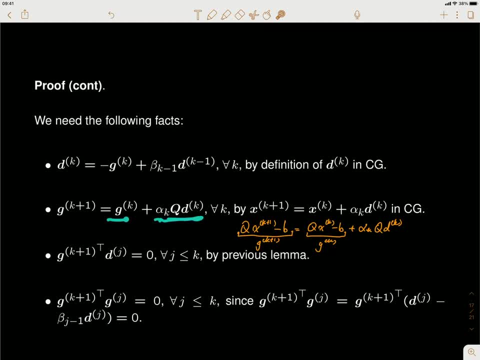 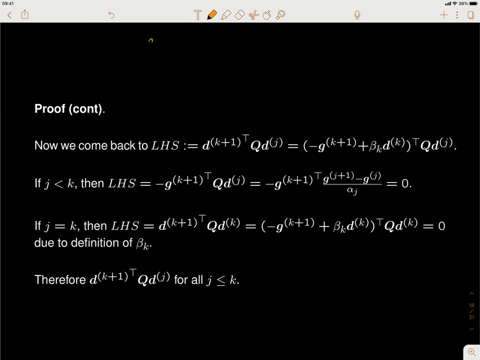 related to the it's. a linear combination can be seen as a linear combination of the g? j plus 1 and g j. Okay, So from here I'm going to get g j plus 1 equals to g j plus alpha j, q, dj. 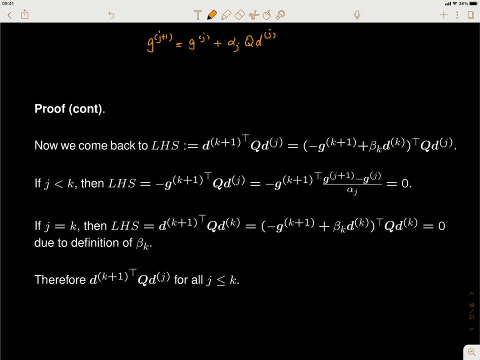 Okay, And then we can just write: q dj equals to g j plus 1 minus g j divided by alpha j. Okay, We can replace by that. The only small issue here, possible issue here is that if the alpha j is equal to: 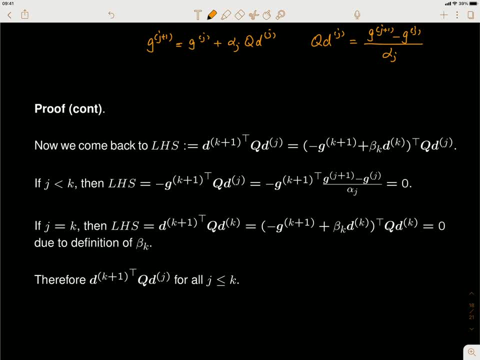 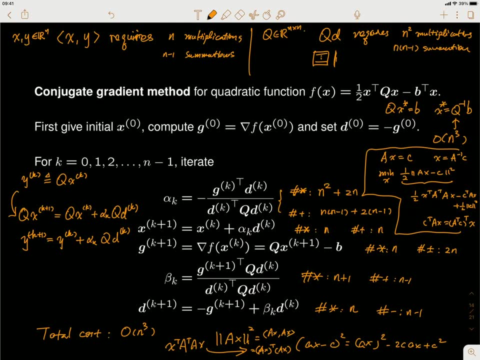 a zero. Okay, What if that happens? If alpha j equals to alpha j, q, dj, then we can replace by that alpha j equals zero. let's see what happens. It means this will be zero, This will be zero, And if this is zero, that means alpha k plus one is just equal to alpha k. 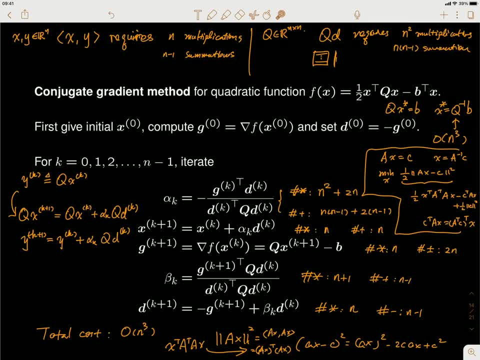 x k plus one is just equal to x k. Okay, the only chance that this could happen is that we already got the solution. We already got the true solution, Okay, and by that time we should already stop. Otherwise, as we said, we'll just keep updating this And as long as we're updating x k. 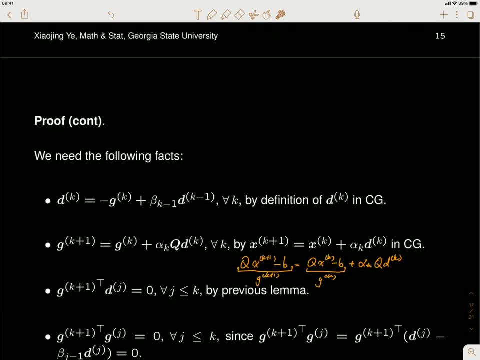 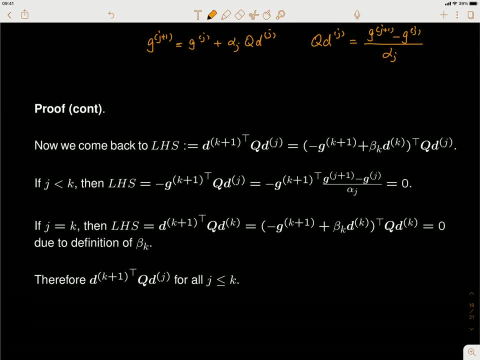 this term cannot be zero, So alpha j will not be zero, So feel free to divide it. Okay, the alpha j will be non-zero And, as we said, we're going to replace the q d j by this, But remember that the j is less than equal to k minus one, So that means the right. hand side can use the q d j. So that means the right hand side can use the q d j. So that means that the right hand side can use the q d j. So that means the right hand side can use the q d j. 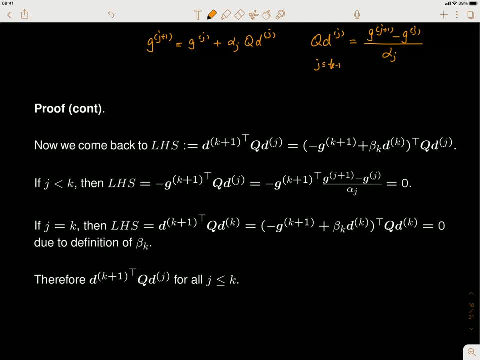 And involve all the j's up to g k. Okay, so this side could be only involved or can be considered as a linear combination of g zero up to g k. Okay, but remember we showed already that the right hand side can use the q d j, So that means the right hand side can use the q d j. 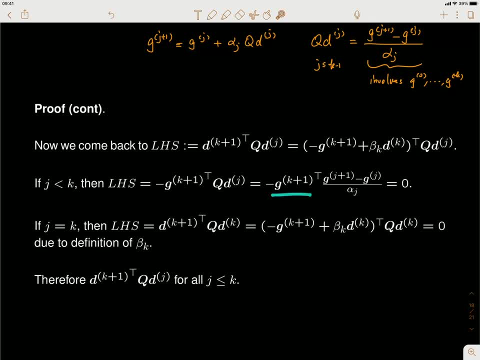 earlier that the g k plus one is perpendicular to all the previous g k's, And now this thing is some linear combination of g zero through g k, And that means this has to be equal to zero. So the inner product of this two has to be equal to zero. Okay, that's the case where j is less than. 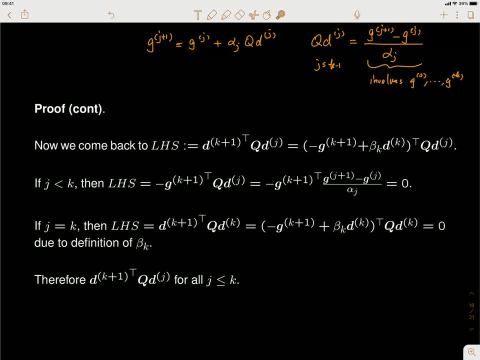 k. Okay, j is at most k minus one. The second case, as we said, is j equals k. In that case, this j is just equal to k. And now we're going to replace the q d j with the q d j. And now we're going. 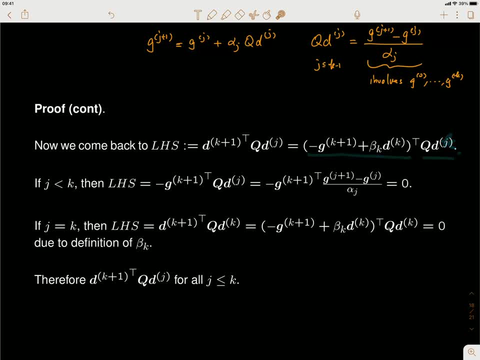 to actually multiply this to d k. So we replace that d k, plus one to this, by this, And then give this q d k here And let's say: if this, let's see this, if this one is equal to zero, Well, 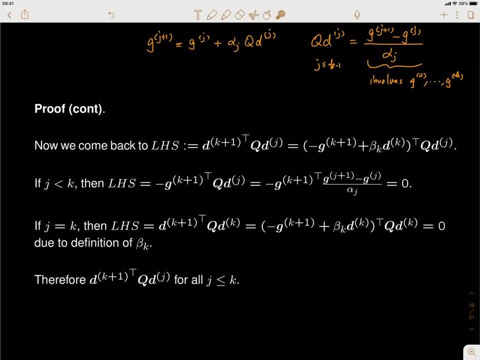 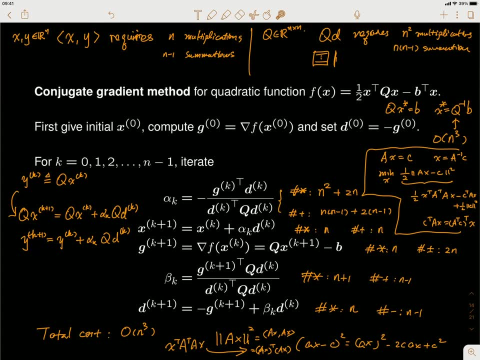 this is exactly the reason why we chose the beta k in the way. as we showed earlier, The beta k was chosen in this form, And that is exactly the uh, the number that makes the combination we saw later as zero. Okay, that's because that's the. 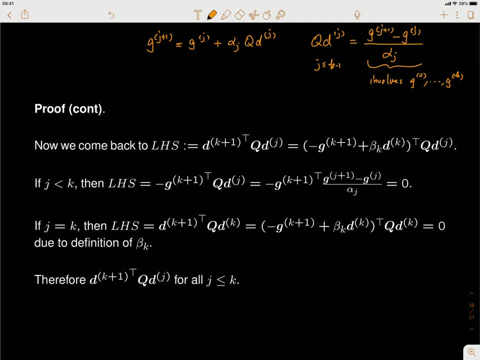 beta k we saw here. So actually we can see this by solving for this beta k, Because we can combine this and this and move to the right, And then we have this thing multiplied to the beta k. So I just need to leave out that number So you can see that is beta k. d k. transpose q d k. 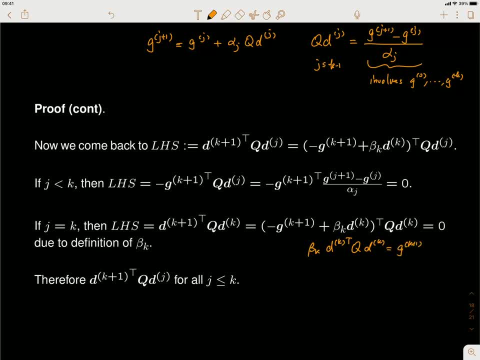 Equals to: I have the g k plus one. transpose q, d k: Okay, and I just need to divide both sides by this quantity: Okay, and again this one is non-zero. The reason is this: q is positive definite And this whole thing will be just the q square, q norm of d k, And unless d is a zero vector. 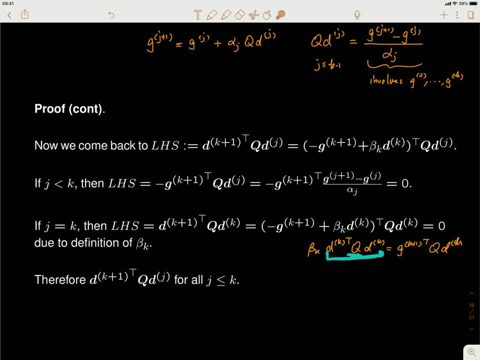 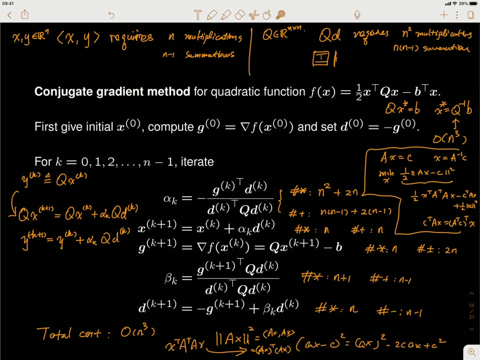 this will be always non-negative. I'm sorry if, unless d is zero, this one is always positive number. Okay, and d cannot be zero. The reason is d is the conjugate direction And we showed earlier that d is the counter direction. It's a linear independent with other d k, So it has has to be non-zero. 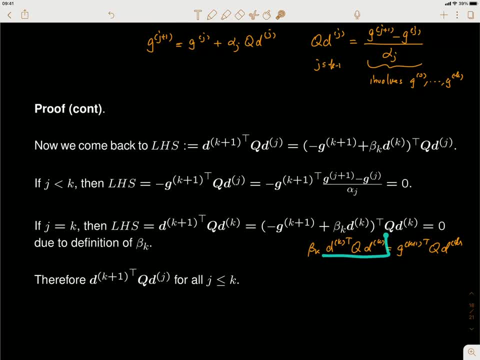 This has to be non-zero. Okay, it has to be non-zero, Okay. so now you can see that we have shown that, for in either case, j is less than k or j equals to k. we can show that this, this quantity here, is equal to zero. 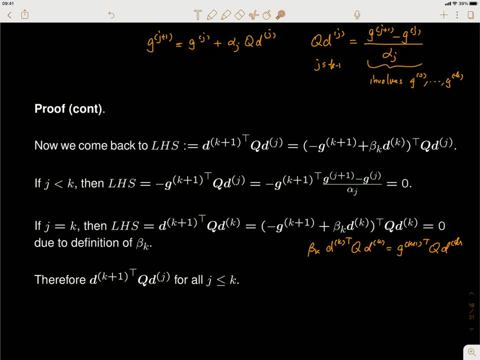 Okay, so I forgot here. this should be equal to zero for all the j less than k, And by this we complete the proof. by induction We show that if d k is d zero through d k are q conjugates be also Q-conjugated with respect to all the previous decays. And that finished the last thing. 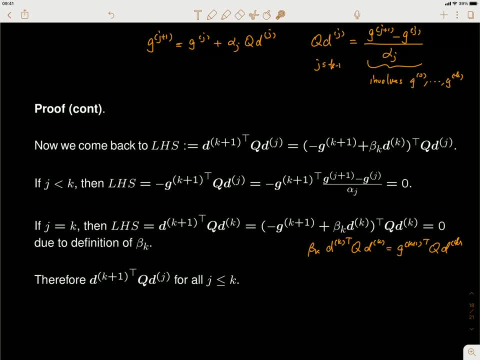 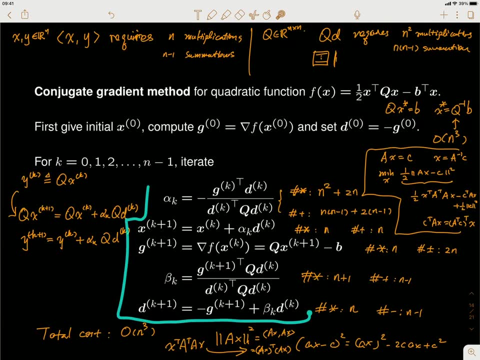 we need for the conjugate gradient method. So in summary what this algorithm is: we need to implement the conjugate gradient method for solving the quadratic, for minimizing quadratic function above here. We just need to iterate the steps here. And the r for k is the. 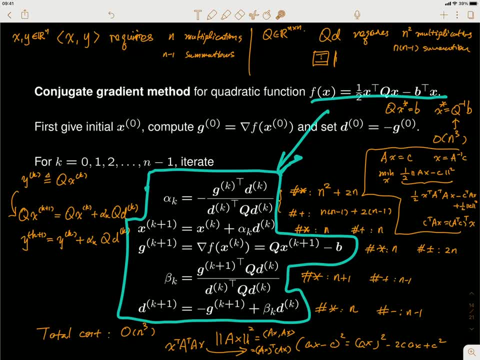 step size. xk is updated from x. xk plus 1 is updated from xk by adding r for k times the descent direction or the conjugate direction, dk, And then we compute the gradient of f, x, gradient of f at xk plus 1.. 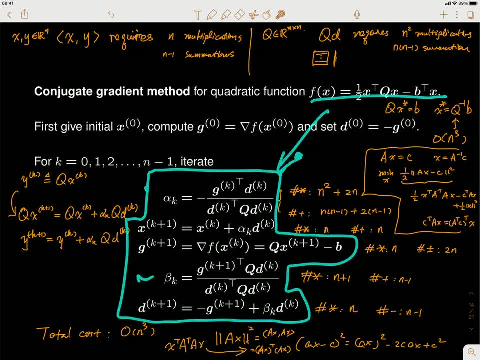 We get the gk and then we compute this parameter, beta k, and use this beta k to get the next conjugate direction. And then we repeat, And we said that the conjugate, these decays, are actually conjugate directions, and according to the property of the basic. 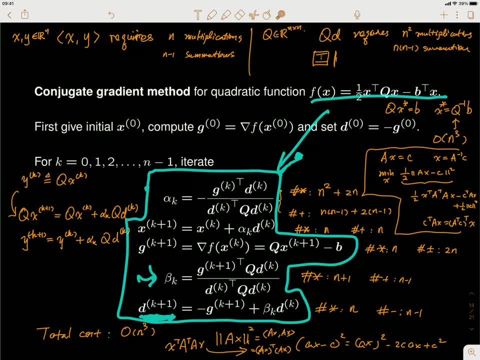 conjugate gradient algorithm we showed earlier. this method will converge within n steps. That means at that iteration n, when x equals to n. this x, n must be a solution, must be the minimizer of this f, x. And that is the latest case. It could happen earlier. as I said earlier, It could happen. 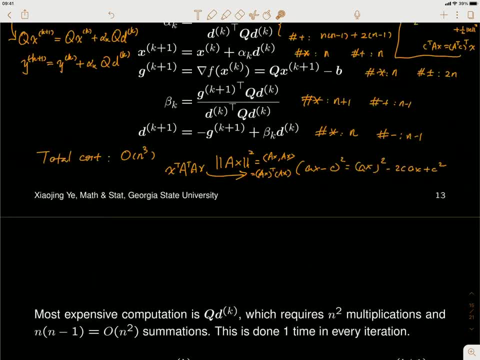 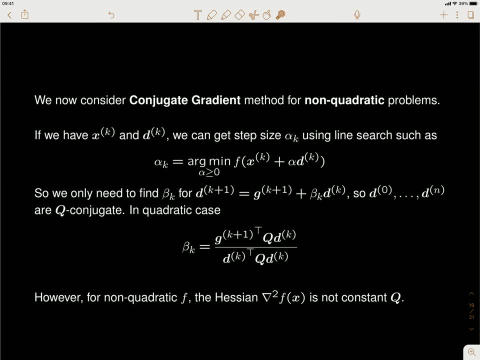 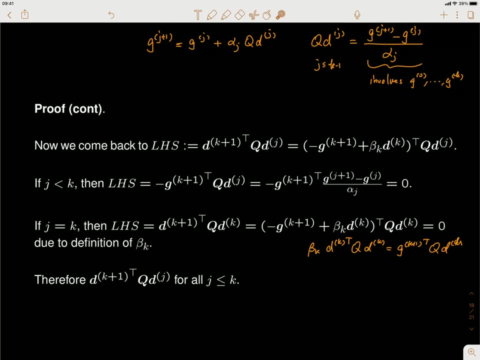 earlier than n iterations. Okay, so this is the conjugate gradient method. So so far we have considered the conjugate gradient method for solving the quadratic function, But in practice it can also be used for solving non-quadratic function, That is. 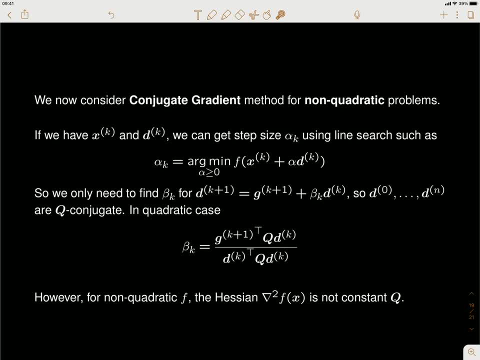 most, actually most more. it's also very common in practice. Not all the functions we're trying to minimize are quadratic functions. Well, if it is not a quadratic function, the conjugate gradient method is not going to guarantee a convergence within n steps. And also, 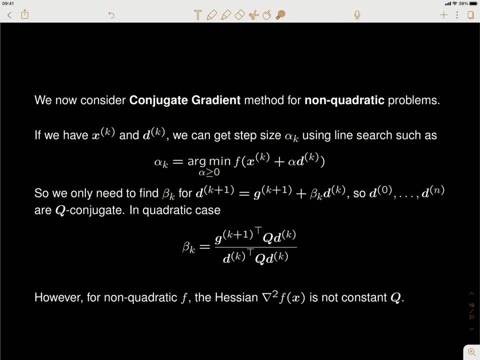 there are some other issues. For example, we are going to: we're going to find the step size r of k And this r of k probably will need a line search because it doesn't have a closed form now. The steeply descent step size doesn't have a closed 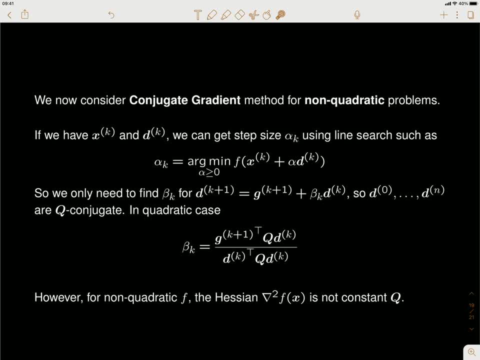 form when f is not quadratic. Okay, and in this case we need to do the same thing as we did for gradient method. We need to use, we need to for every x, k and d k. given x, k and d k, we need to find this alpha. 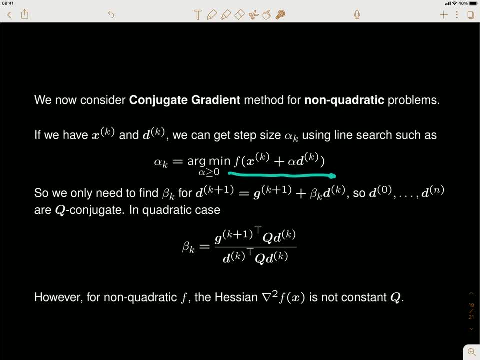 by minimizing this line search function. This is the function of alpha, a scalar alpha. So we can use a secant method or something like this, like that, to solve for this minimum, to solve for the best step. size r of k. Okay, and also, the beta k does not have a closed form. 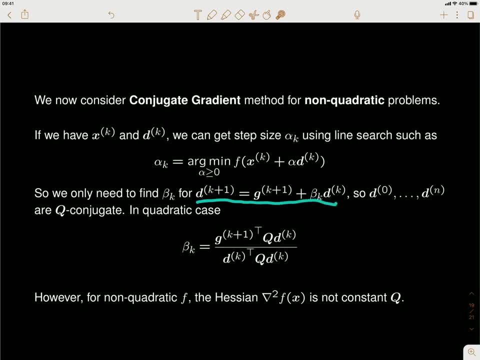 for that either because previously we got the beta k when the function we're trying to minimize its quadratic function, And then that's how we obtain the beta k. But here I think it will be a negative here. But here the issue is that it's not a quadratic, So we don't really have the beta k. 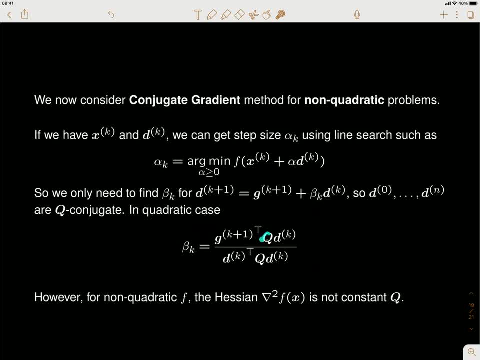 formula like this one, because the q is the q in the quadratic function, but it's not a quadratic function. this q is changing every time, right, because this q is actually somehow like the Haitian matrix of the function f at the point xk. 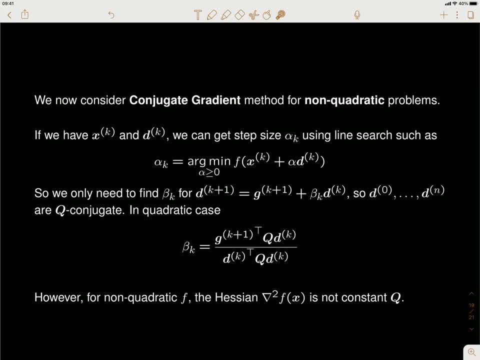 and that's changing, So we cannot really have this beta k formula, okay, while I set it here. So if it's a quadratic function, the Haitian. so we said: if it's a quadratic function, f equals to one-half x transpose q minus b transpose x. we know that the gradient 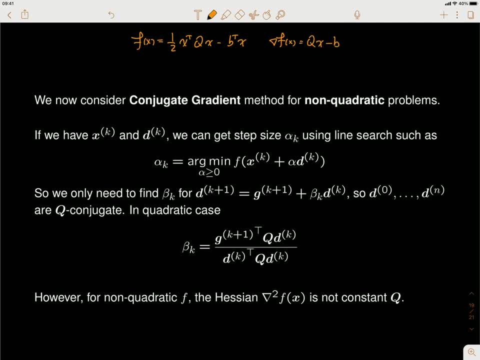 f is clear, which is just xk minus b, and the Haitian is just q. But if it's not a quadratic function, the Haitian may not be a constant q matrix. It could be changing. Okay, now what happens? what we should do in this case? There are several ways to modify the. 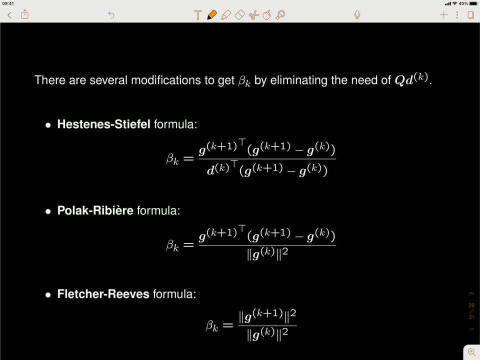 formula for the beta k so that we can still update the beta k. Okay, and the first one is called Hastenitz's default formula. So what they do is to try to get rid of or try to limit the using, avoid using this q, dk. So if we said that the q is changing every 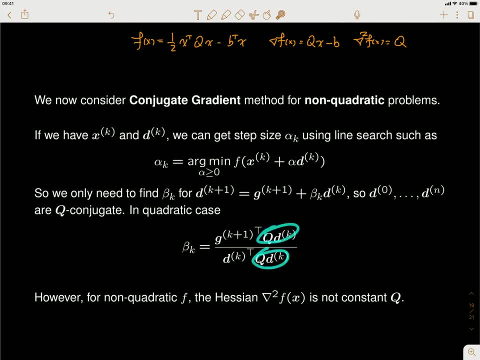 time. Okay, so they, they, they're trying to avoid using this q dk. Okay, so they, they're trying to avoid using this q dk. Okay, so they, they're trying to avoid using this q dk. Okay, so they, they, they're trying to avoid using. 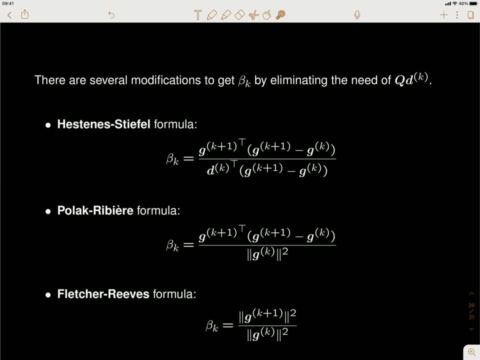 this The first, first way, first formula Hastenitz's default method is replacing this q dk by this, by this quantity, And this is it has some. it has some motivation because we previously we showed that for for the quadratic case the g, k plus one was related. 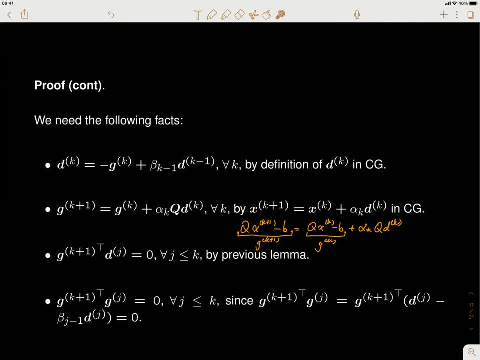 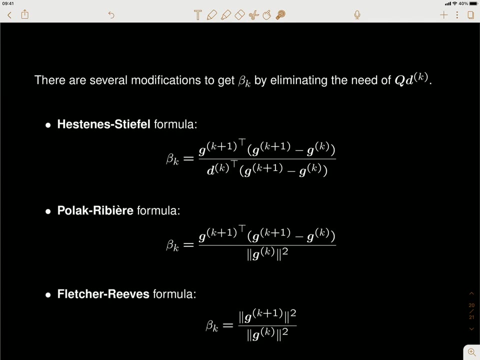 to. so I hope you can still remember the q dk was related to q dk and that's what qdk is equal to, this minus this divided by alpha k. so now i have a qdk on both numerator and denominator, so i can replace that by this gk plus one minus gk, and that is the reason why i've had 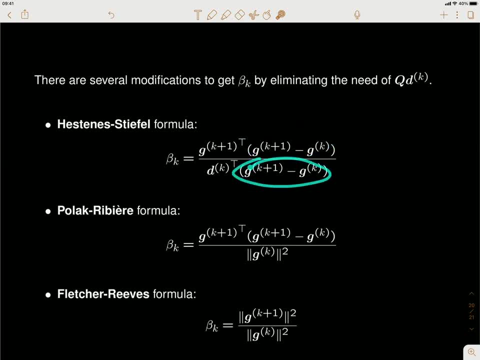 this one here, okay, and also the denominator is replaced by this and the two alpha k's are canceled. we cannot really cancel this vector with this vector, because we're going to multiply this vector to another vector is the inner product, so we cannot really cancel this two. but the alpha k, which is scalar, it can be pulled out and it can be canceled. 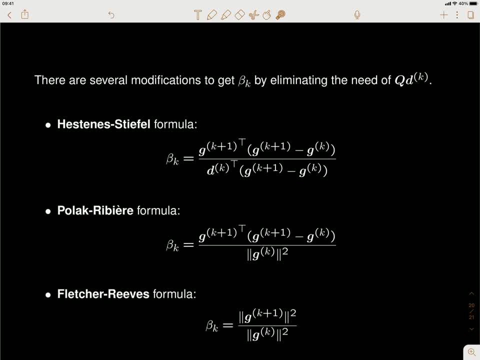 okay, so that's the first formula. the second is a polyrheumic formula, that is, the numerator doesn't change, but the denominator is replaced by the gk square. okay, it's replaced by the gk square. um, that's the second formula. the the third one is the fletcher reeves formula, and that's also. 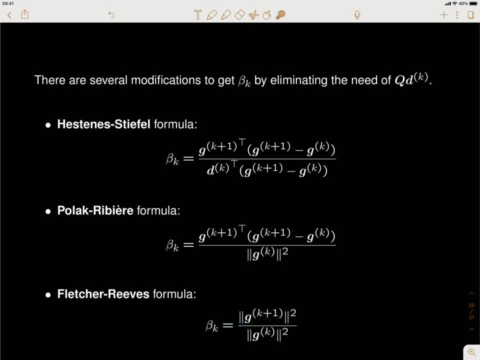 replacing the numerator by the gk plus one squared. okay, so they are all uh kind of replacement for the original formula, uh, in order to avoid using the dk, qdk, but uh, they all reduce to the same formula using. they all reduce to the same formula, like this one, when we're actually 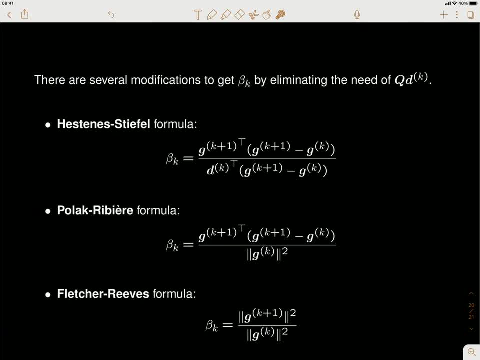 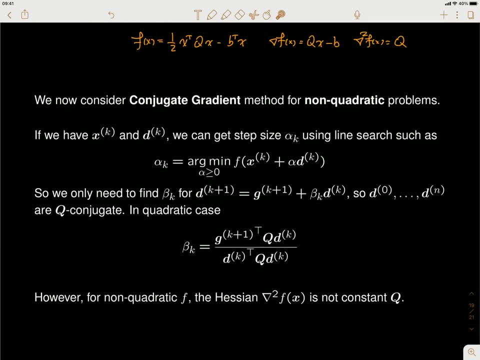 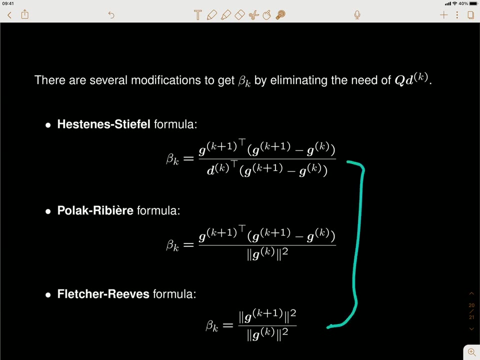 working on quadratic functions. okay. so these are all generalizations over of the of the formula here. okay, so what i'm trying to say here is that if you are really working on a quadratic function, don't worry, these three of these three will reduce to the. the formula here will reduce to. 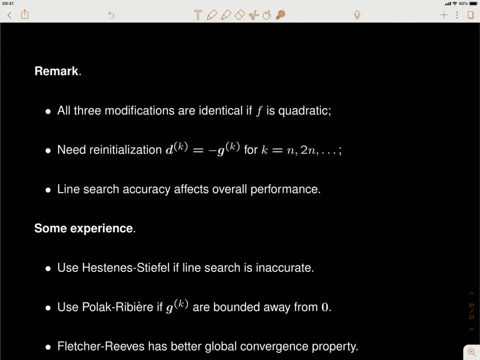 this one, okay, and uh, some uh remarks. um, so i said the first, when all these three modifications or will will be reduced, will reduce to the original one, original country reading method when f is quadratic. so they still want to keep the optimality of the country reading method when applied to. 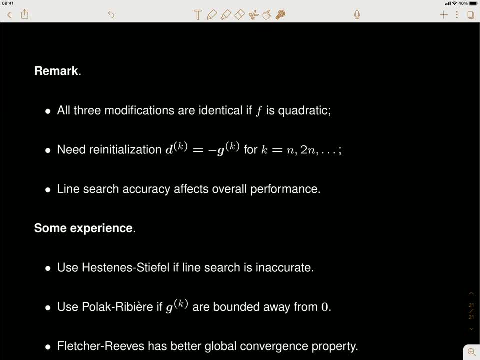 quadratic function where, which is the one original purpose for the development of the country reading method, uh. second, is that um? since it cannot guarantee convergence within n steps, we probably expect to run more than n iterations, and uh, it is usually. we need to do this so-called 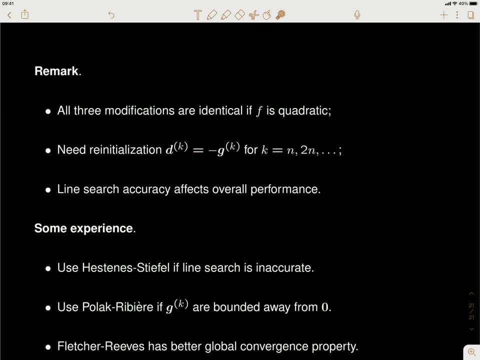 reinitialization of the dks, because uh, after k or after n iterations, where n is in uh, the, the dimension of the problem or dimension of the x, uh, we probably run through all the concrete directions. so we need to reinitialize the dk to the current negative of gk and repeat the procedure. 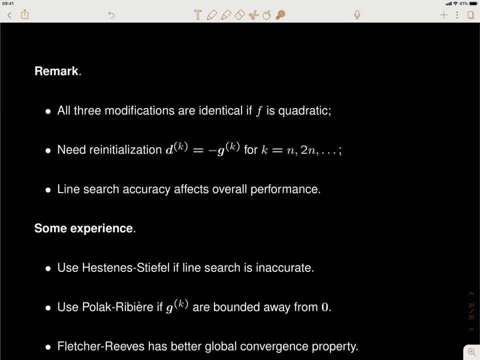 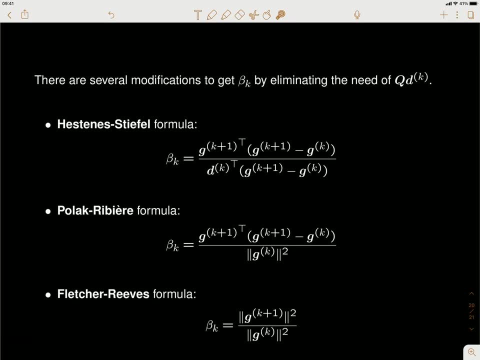 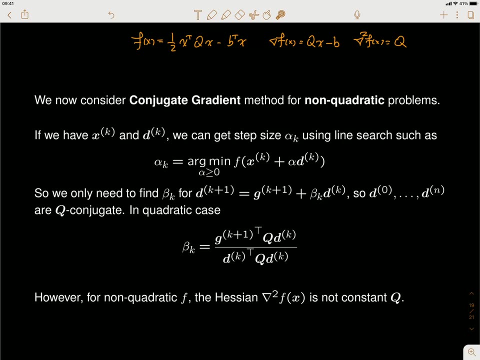 okay. so that's why uh reinitialization may be may be required and also the line search accuracy will affect our accuracy over our performance. this is line search accuracy. you can do it very accurately, but it's expensive to do this. but i need to find uh, the optimal alpha and that. 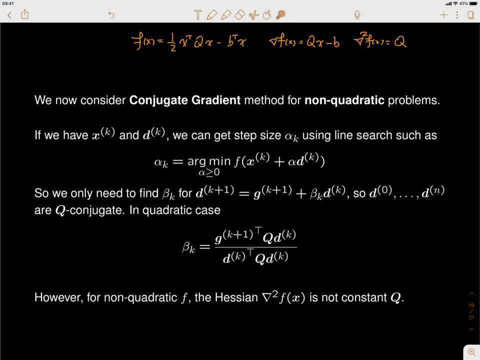 requires taking the gradient of this multiple times. that can be expensive. uh, actually, you can show that taking the gradient of this requires a q times. this q times is minus b and the q times is: it's a matrix vector multiplication and that is n square of the computation general that can make us expensive. 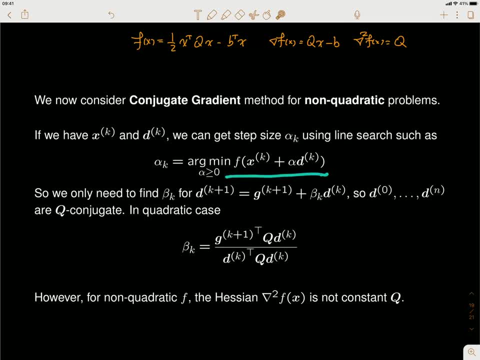 so you can either spend more time on this and hopefully you can get less before iterations, or it can be a little bit less accurate here and you can just run this second method for a few iterations. but hopefully that after you update this r for k you can immediately move on quickly. move on to the next point. 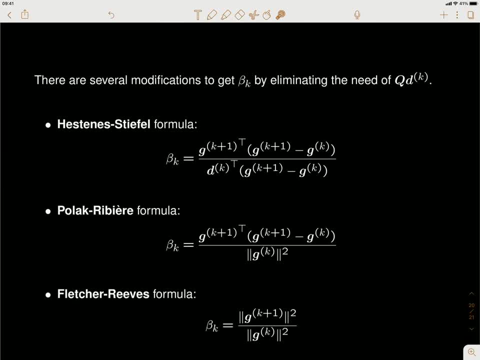 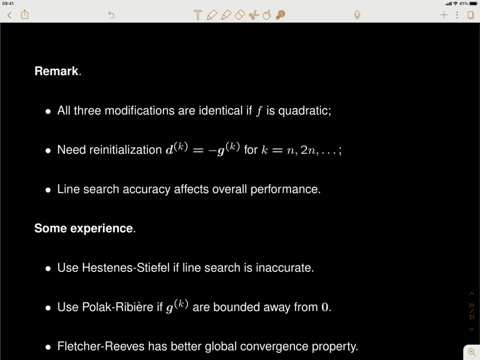 and compute the new uh descent direction or country direction and that probably can help uh improving the overall performance, because i've said that overall performance is not only the total number of iterations but also the uh computational cost you spend for each iteration and uh the line search takes some computations for each during each year. so 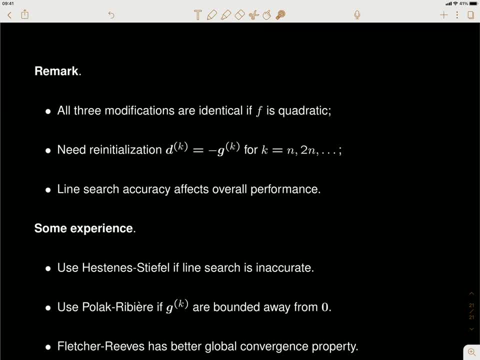 you want to keep that computation complexity low? uh, okay, uh, in some experience when you use this algorithm, surely there are are very mature uh software packages in python or my lab or even other uh softwares, so they all implement these methods and you, you can use the hesitantness. 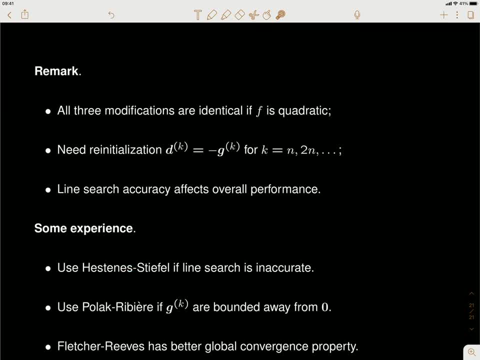 default method when the line search is not very accurate, and you can use this one when the gk is bounded away from zero, and you can use the flasher reefs method for better overall convergence. so you can try all of them in practice. okay, so this completes the discussion on conjugate gradient method. 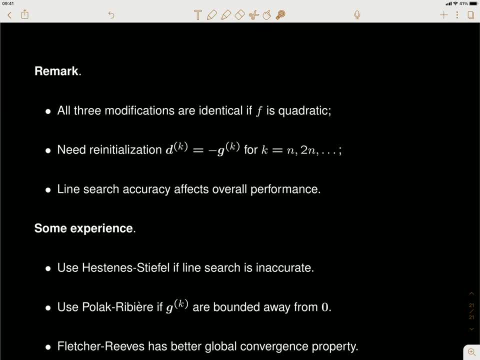 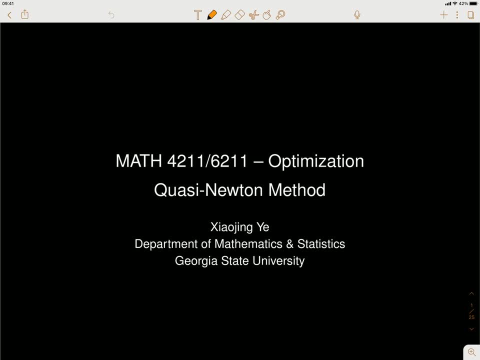 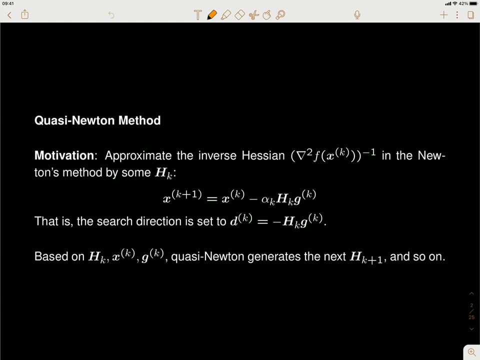 okay, next we're going to talk about a important, important class of optimization methods called quasi-newton method. so the quasi-newton method is a modification of the newton's method. so before that, we first recall, the newton's method was set to this update rule. the x, k plus one is: 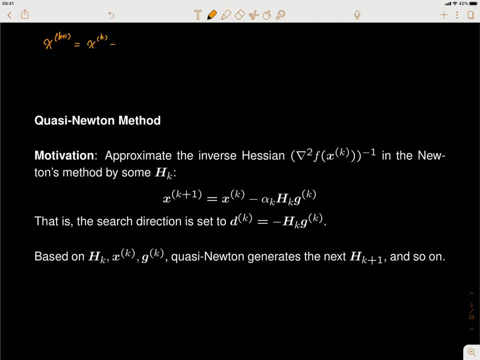 computed or is updated from x k by doing this operation. this is a h of f at x k plus one, so x k, and you need to take the inverse of this and then multiply to the gradient f at x k. okay, and this we usually call it h k. okay, this is a h of f and x k. this is the matrix m by m matrix. this we usually 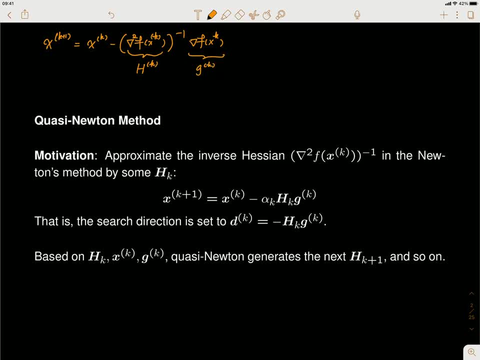 just denote it by g, k, which is m, by one vector is n dimensional vector, just like x. okay, so this is newton's method. well, what is quasi-newton method? um, this is trying to overcome the issue with the newton's method, because in newton's method we need to compute this thing. 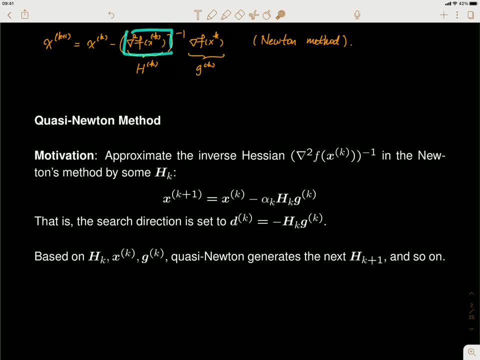 and taking the inverse of this matrix, or at least we need to solve, we need to solve for the vector, so we can call, say we can call this whole thing to be to be the- uh, negative decay, okay, and then we need to solve the negative decay from the 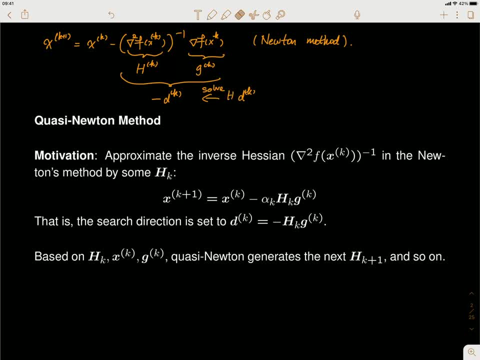 h k. sorry, let me just try to reset this part. so I'm going to solve the d k from h k. d k equals to negative g k, so suppose we are at x k. we can compute the gradient g k and the h k and then to solve for the vector d k. 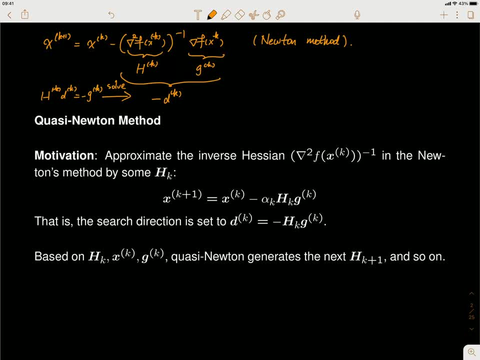 and uh, that's my uh d k del h dk will be. by solving that, my dk will be equal to h k, negative h k, g k, or in other words, negative dk will be equal to h k times g k. okay, and usually this is how we get this vector and then, once we 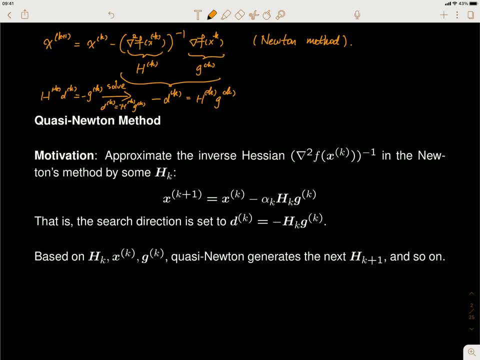 have that we can subtract the dk or minus dk from the xk, so that will be xk plus 1 equals to xk plus dk. okay so, but anyway, the key is to solve this linear system, and that solving this linear system is not easy, as we showed before we, the country agreed in the matter, was almost dedicated to. 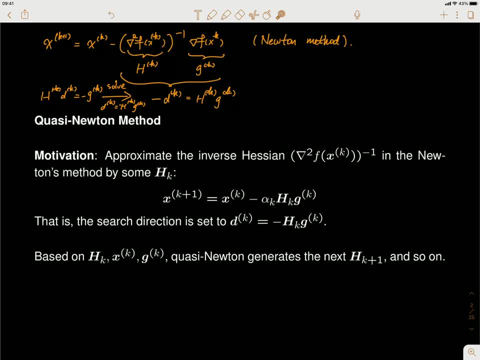 solve this kind of problem because this could be very large matrix okay, so solving a universe of this matrix not really practical in the real world. so that's why the nudist method is not really popular in practice, although it has very nice convergence property we showed before it is and it's converged at an order two and 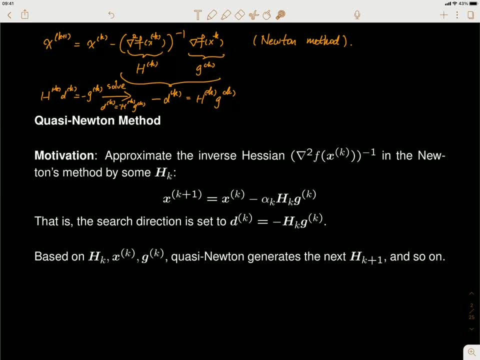 let's say it's considered as a very fast convergence, but the per iteration cost is too high. i need to spend lots of expense computations for each iteration and that is a drawback with the newton's method. and there are several other drawbacks with newton's measure we discussed. 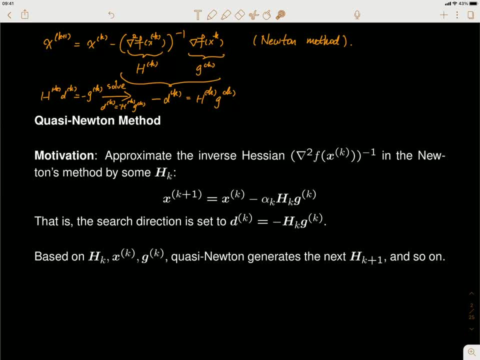 earlier, but this one appears to be the most difficult one, okay, and that's why people came up with this quasi-newton method- is trying to approximate the inverse haitian. remember, the inverse of this haitian matrix is the most troublesome term, okay, or this term, this is: 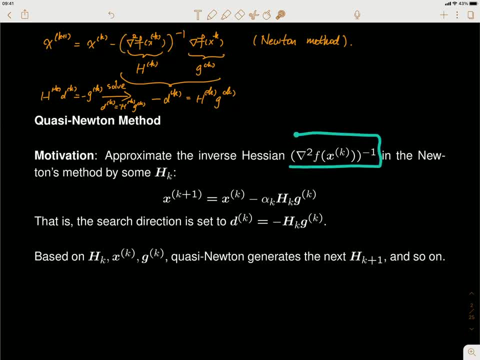 the most troublesome term. so we replace this inverse of the haitian by some hk. so this hk, you see the notation. this hk is different from this hk. we'll have the superscript k, that means the haitian matrix. so once you get, once you have the xk, you can compute. 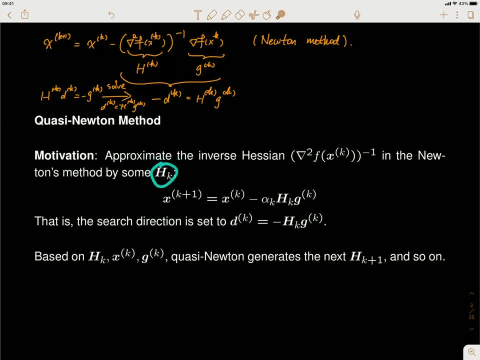 the haitian, but this hk is some matrix that we can, you we're using to approximate the inverse of the haitian. okay, so, uh, if we can really do this, then our update rule will become very simple. the xk plus one will be updated from xk minus alpha. k is the step size and this hk. 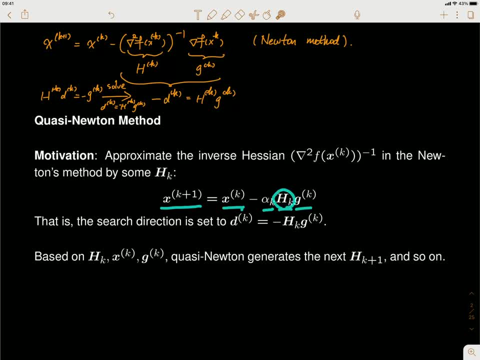 the gk is what we had earlier and this hk. if we were using the haitian inverse of the haitian, then this just becomes the newton's method. uh, if we further set alpha k, step size, alpha k to be to be one, but right now we're replacing this haitian inverse of the haitian by this hk matrix and the 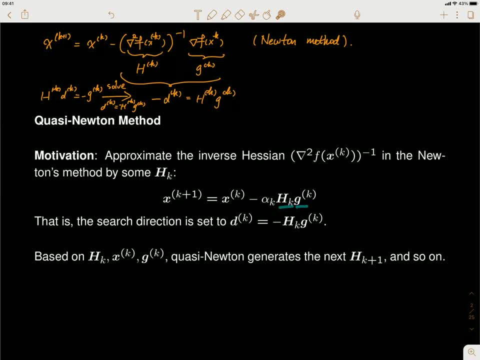 hk. we multiply these two. that's simple. it's just a matrix vector multiplication. that's supposed to be simple, okay, uh, or in other words, we're actually doing the standard gradient descent method with this step side, with this search direction, dk set to negative of hk, gk. okay, so the key is in this hk. 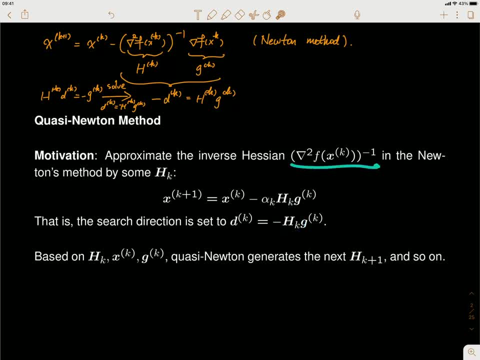 how do we get this hk so that it can approximate the inverse haitian? okay, and if it is- uh, you can find a very good approximation- then this method is potentially, can potentially behave, similar to the, to the newton's method, and that means it can convert really fast. 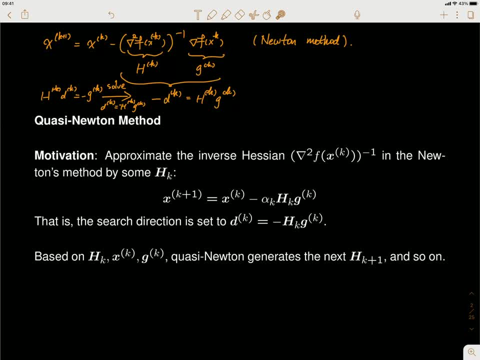 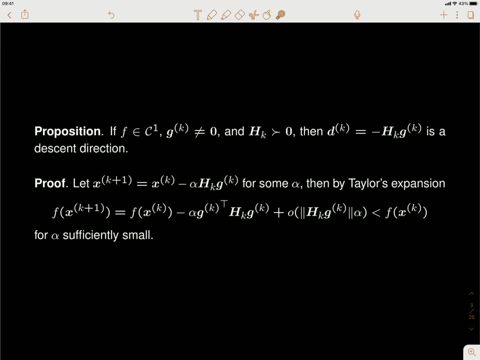 okay, so that is. that was the motivation for the quasi-quasi-newton method. and now let's see why. well, what is good for this? what is good with this kind of step size? the first thing is we call that the. it is equivalent to a gradient decent algorithm with dk, decent direction, dk set to negative, hk, gk. 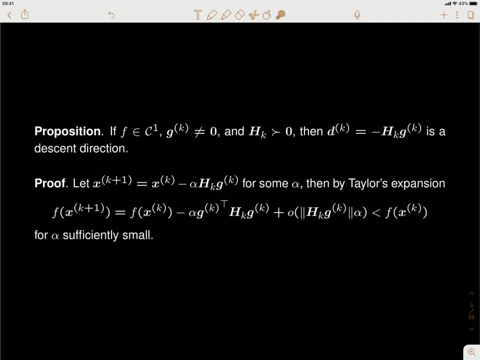 if this hk is positive, definite, then this decay is guaranteed to be a decent direction. and the reason is that, uh, remember, for this dk to be a decent direction, we just need to show that, for step size, alpha, alpha, small enough, going along this direction will give us smaller function value. 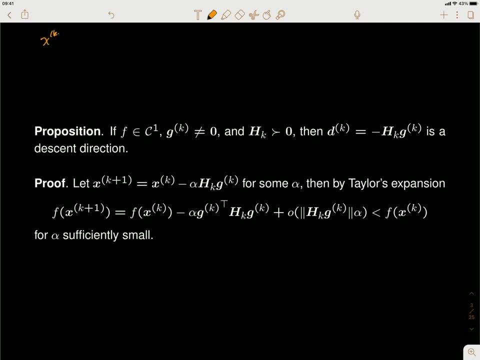 right, so we'll say that i have an x k plus 1 equals to x k plus alpha dk. okay, it's a decent direction or it's a decent? it's a decent method if f of x k plus 1, according to the definition of x k plus 1, is just f of x k plus alpha dk. 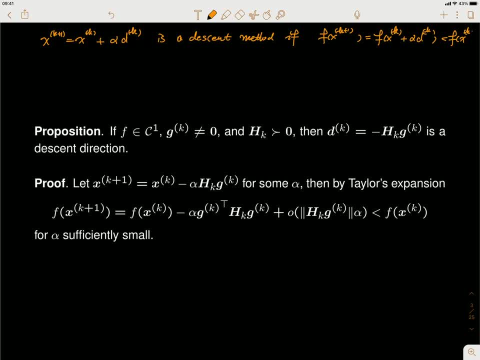 is smaller than f of x, k, when this alpha is not large. right, that means your next point will have a smaller function value than the previous one and that makes this function value decreasing. and that's that's basically aligned with our goal to minimize the function f. okay, and here, if we set dk to be negative, hk, gk. 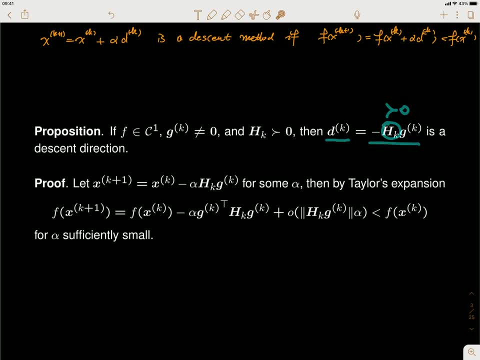 with positive definite matrix hk, then it's guaranteed to be a decent measure. okay, that means this will happen and to show this, we have seen this uh kind of proof before. to show this easy, you just define the line search function phi of r alpha, which is such as a function of the scalar alpha. 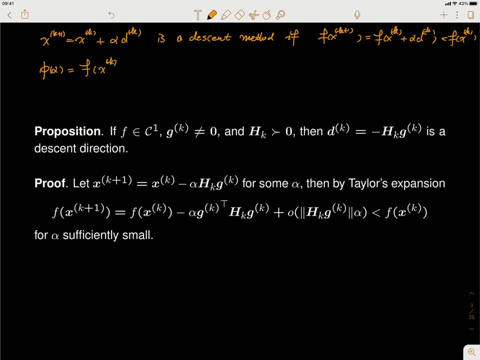 and then we set this to be f x k plus alpha dk, okay, and then the phi zero will be just the f of x k and uh, if we draw the picture of this phi, this is the r, this is the alpha, this is zero. so this is the phi of zero and this, basically, we're looking for the function value. 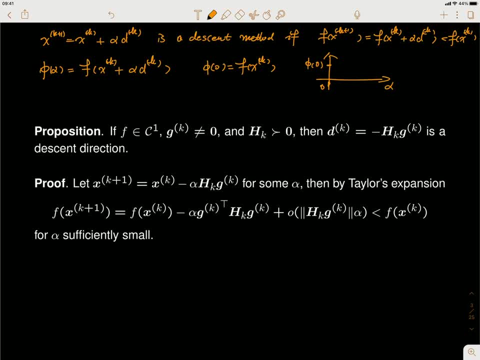 along the line from starting from x- 0 or along the array uh, starting from x k, and go along the direction dk and the step side, alpha is the step size. so we go along the direction. if we can show that the derivative is negative at this point, then, uh, it will go go decent, like this and maybe 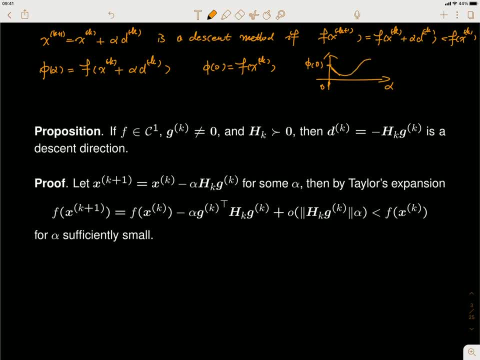 eventually you'll go up, but we don't care, at least for alpha. small enough, the function value should be decreasing, okay, so the only thing we need to prove is to, to, to prove that the f, the phi prime, is equal to zero, as zero means. we need to prove this: is is smaller than zero. and the question is: if this is true, okay, so 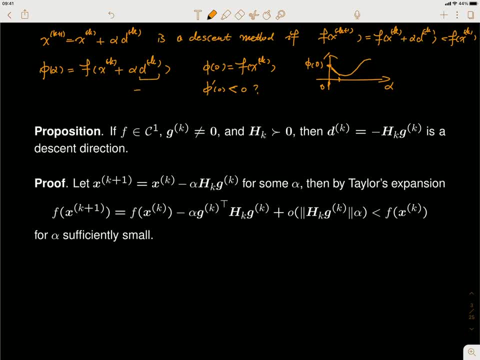 recall that our dk was set to negative hk gk in the quasi-newton method. and now to compute the phi prime of alpha. we have done this many, multiple times. this is just the gradient f of x k minus alpha hk gk, since this is our dk now, and then we need to multiply the derivative. 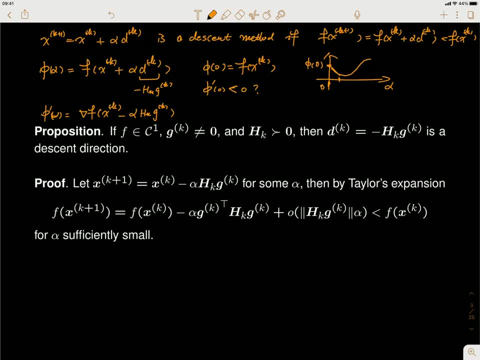 of the inside with respect to alpha, due to the chain rule and the inside multiply what is multiplied to alpha. let me just replace this. this is actually just a negative of hk gk. so when i multiply the grid, multiply the gradient of the inside with respect to alpha, i will get 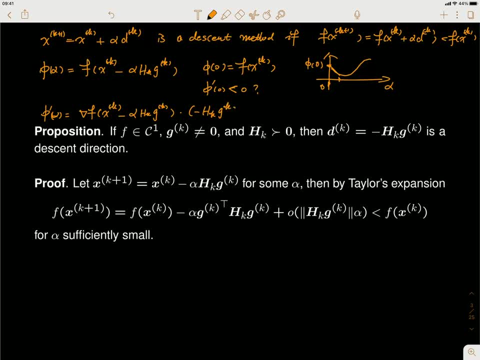 negative, hk, gk. okay, and now we can see that. what is phi prime at zero? we just need to set alpha equal to zero. but the alpha equals zero means this one here is just zero. okay, so that's what we're going to do: to set to zero there. so 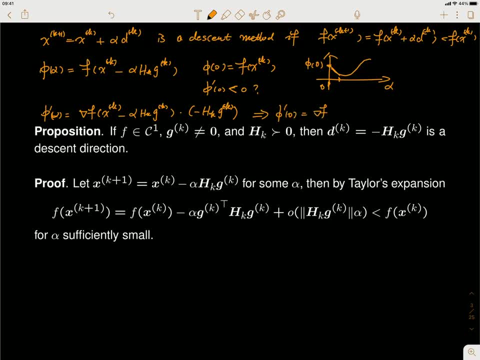 phi prime at zero is just a gradient f and xk. now this becomes zero times negative hk, gk. okay, i pull out the negative and realize the green f at xk is just gk itself. i have just gk transpose h, gk, hk, gk. well, as you can see, if hk is positive, definite. 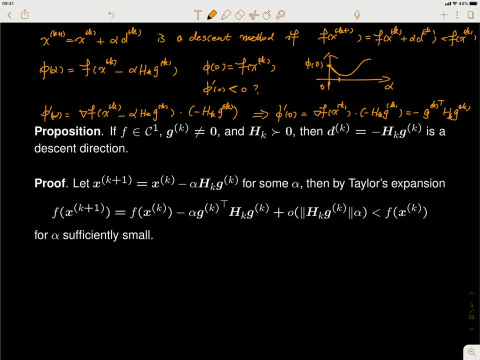 and g is not zero, g is not zero. watch, even if g is zero, already reached to the, at least reach to the critical point. and they already give us the solution: our local minimum or something like that. so we, we, in practice people, you really stop, just stop there. so, uh, but if it's not zero, 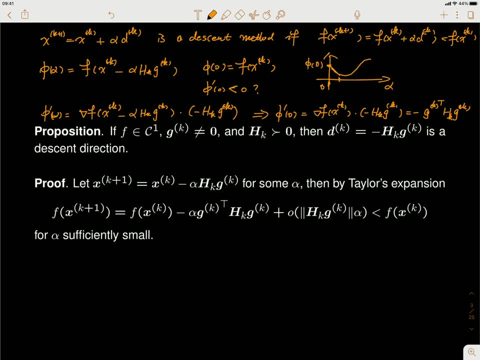 that's when we can still make progress. but when gk is not zero, hk is positive. definite, that means this. so the proof i gave here is that the gk will be strictly positive and the negative of this will be strictly negative. so that's how we show that the phi prime at zero will be negative. 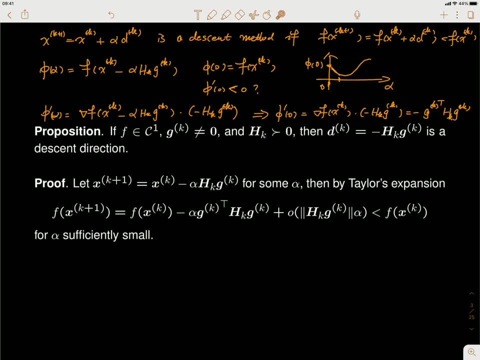 if the hk is a positive, then definite matrix. so that is also one of the principle that we want to follow when we design the quasi-newton's method. we want to set up this hk so that it's always a positive, definite matrix. so the proof i gave here is just the same, exactly the same idea. it just uh express out what this. 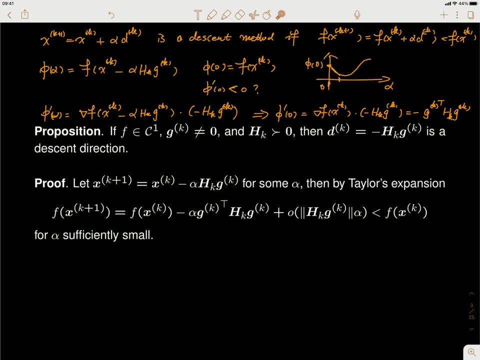 line search function actually is, and from there you can show that by realizing that xk plus 1 is just xk minus this. so i can take the tailoring expansion of this f, because this xk is nothing just like this. so i expand this. at the point xk i'll get these terms and if i want to kind of break this, I can just look at the several examples. so if f is an 810ANA, 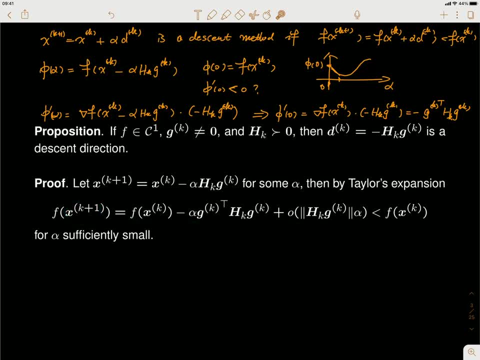 to see if it is an 810 xk, and then we need 810 to find the�'s spread going, not just these 3, 5 and 6, because this xk, xs is nothing, just like this. so i expand this: at the point xk i'll get these terms and if i want, 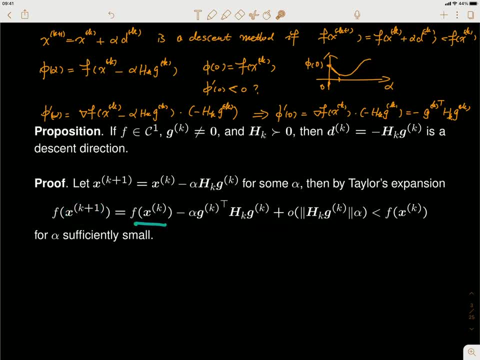 want this whole term to be less than so. this is the zeroes order term. this is the first order term. you can try it by yourself. it's just the first order term. this is the second order term and it is supposed to be little o small o of alpha. so that means if alpha goes to zero, this term will. 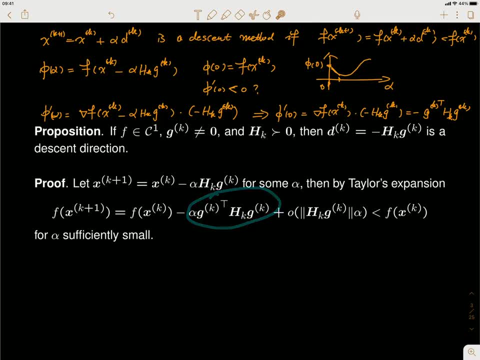 go to zero faster than this term. okay, and so if you want this whole thing to be less than f of xk, that means you want this whole thing to be less than zero. you can just show that this part is positive. if this is positive, then when alpha goes to zero, this whole thing will be dominating. 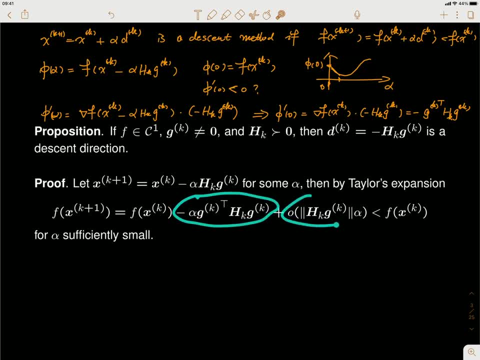 this term will be a negative term that is dominating this term and that will make the sum is two circle terms less than zero and that will make this smaller than this. f of xk. okay, so this, okay is just this: just make this is less than zero and uh, when? when the hk is positive, definite if gk is non-zero. 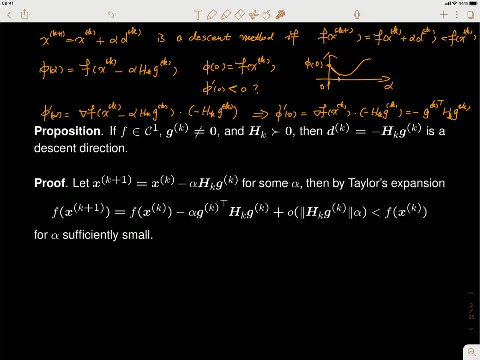 then this is guaranteed to be, uh, strictly positive. okay, and that's. it has exactly the same idea as used in my in my written proof. 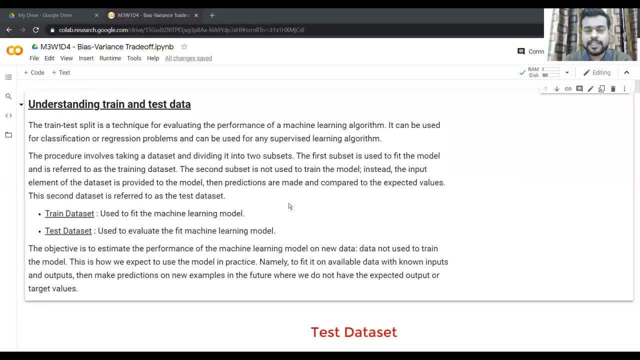 Today is also a very important technique which we will be discussing, and mind you that this technique is not limited to linear regression, but it is more or less a general modeling technique, or in fact, yeah, so it is sort of pervasive across different algorithms, which we'll see especially in supervised learning algorithm. So, yeah, so that's what we're going.